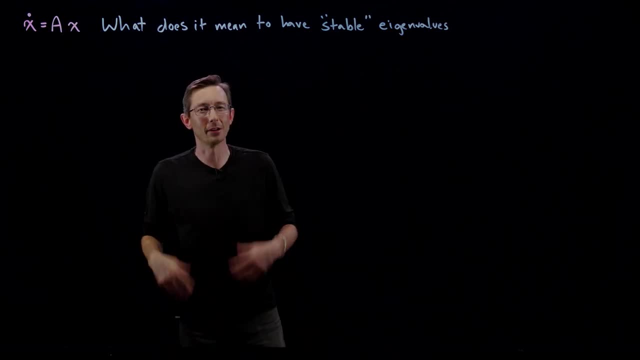 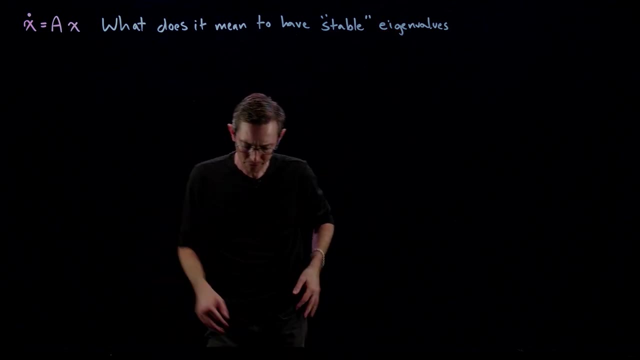 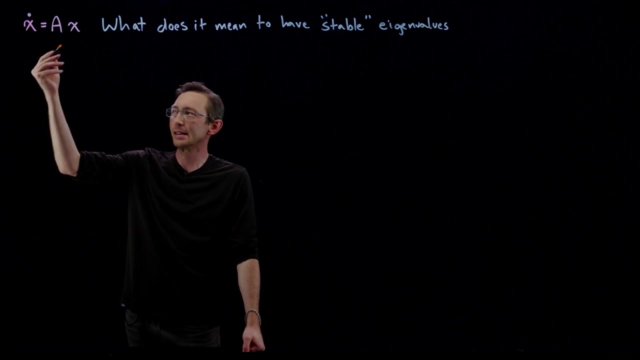 I like I use this phrasing all the time and I realized maybe you don't know what I mean when I say the A matrix has stable eigenvalues. So I want to just dive in and make it very, very clear. We know, for example, when we talk about stability- if I talk about, you know a really simple 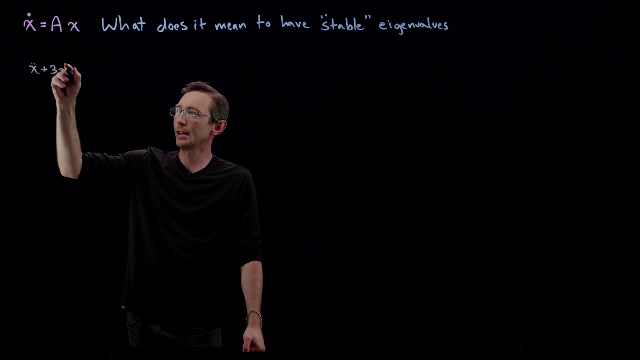 equation like x double dot plus three, x dot plus two x equals zero. we know that the solutions of this differential equation are things like you know: x of t equals. there's two fundamental solutions you can find from the characteristic polynomial And those two characteristic. 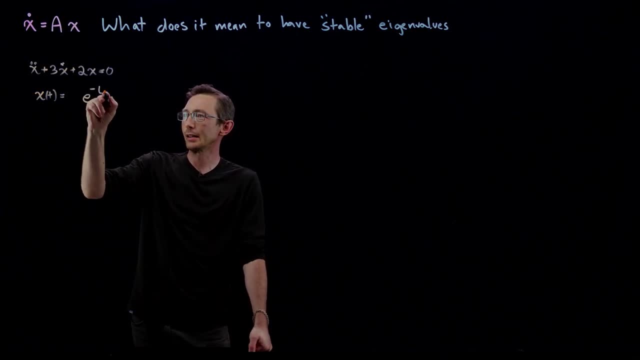 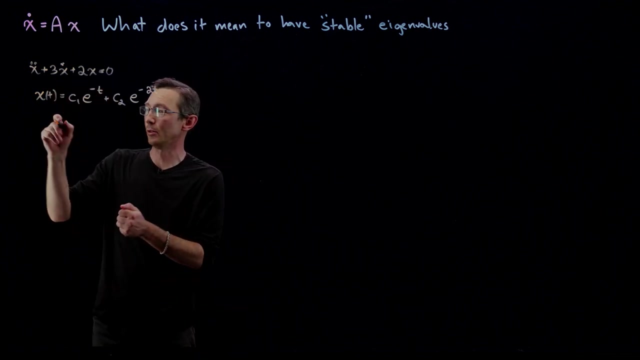 solutions are e to the minus t and e to the minus two t, And so any linear combination of these two solutions is all-in-one. So we know that the solutions of this differential equation are also a solution to this differential equation And we would say that this system is stable. 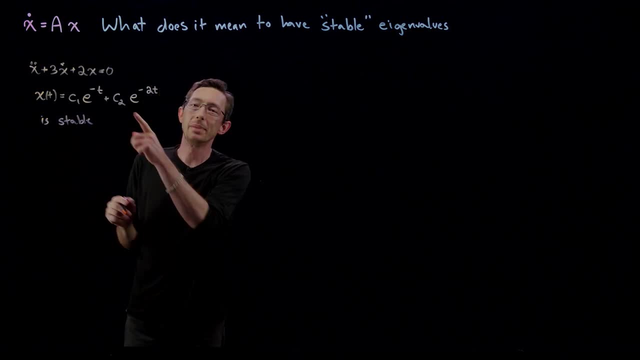 is stable because all of the fundamental solutions are stable, exponential. It's stable because all fundamental solutions, kind of- in this case there's only two fundamental solutions, but all the fundamental solutions- e to the minus t and e to the minus two t- are in fact stable. And literally what that means is, if I plot these functions as functions of time, 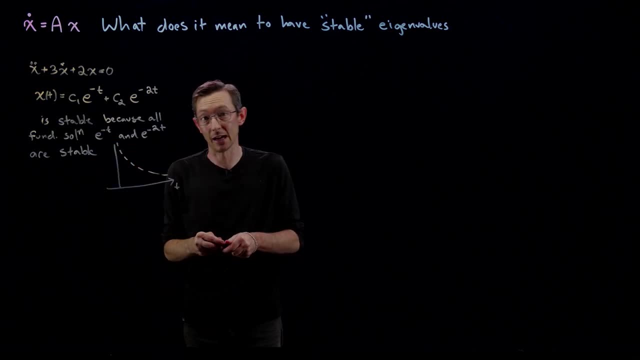 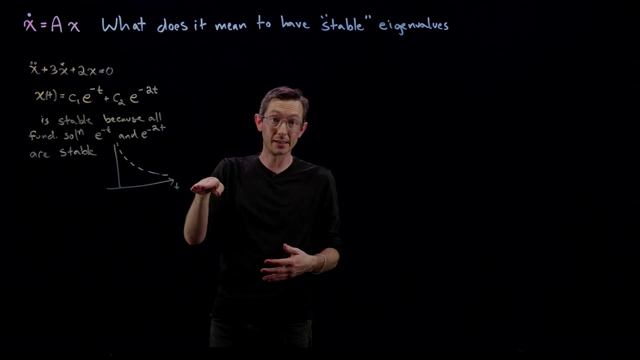 they are decaying exponentials. They decay to zero as time goes to infinity. So this is stable because the solution goes to zero, It remains bounded and, in fact, converges to zero asymptotically as t goes to infinity, as time goes to infinity. So that's what it means for this to be stable. 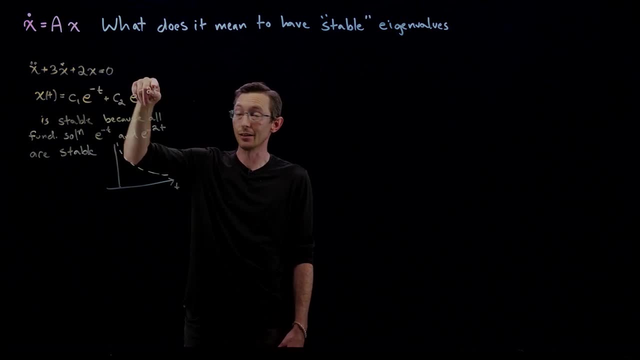 is that all of these powers of e to the minus t and e to the minus two t are stable, And so e to the minus two t are stable. They have negative, they're negative- real numbers. So e to the negative real number t is going to get, you know, arbitrarily small, as t goes to infinity. So how? 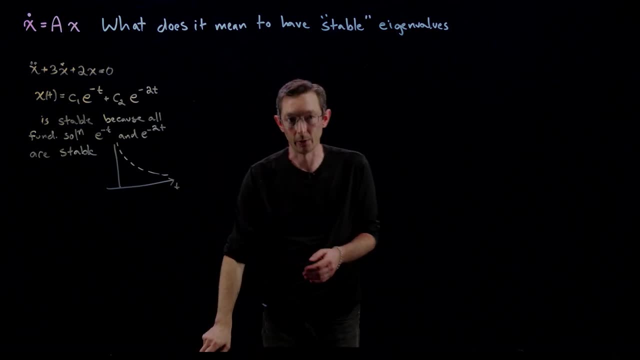 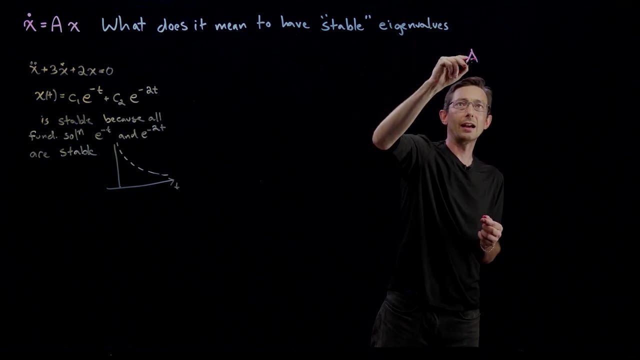 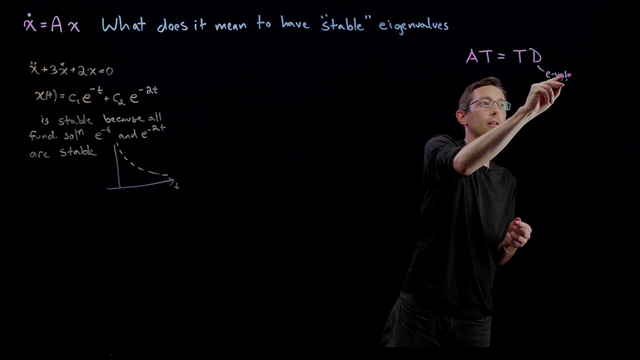 does that translate over to these matrix systems of differential equations? Well, we know, in this matrix system we're going to be talking about things like eigenvalues and eigenvectors. So we have a times t equals t times d, where these are my eigenvalues and these are my 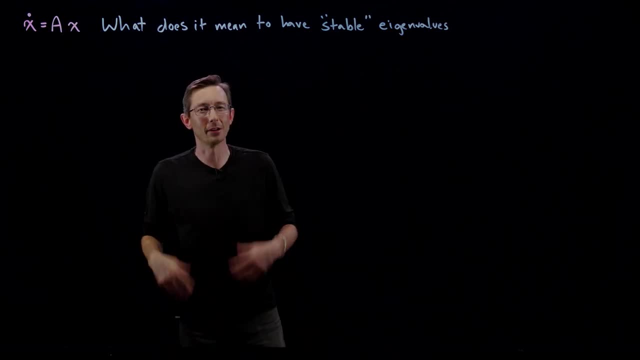 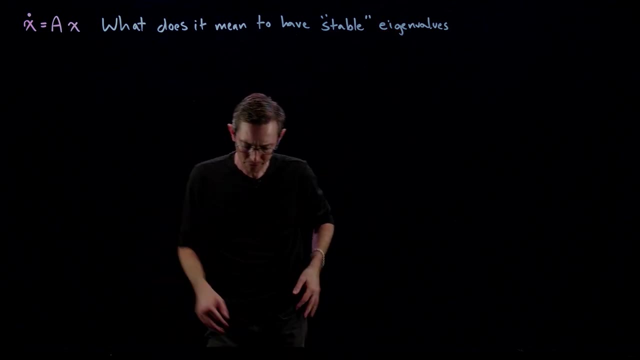 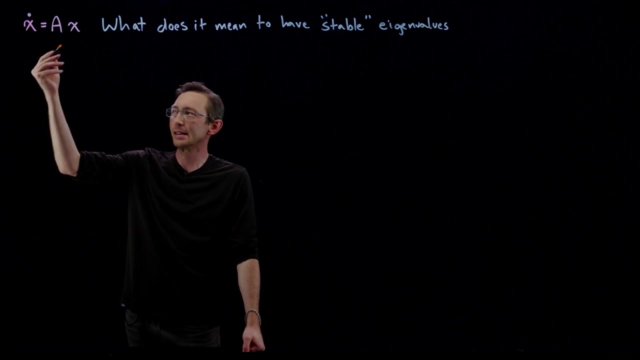 I like I use this phrasing all the time and I realized maybe you don't know what I mean when I say the A matrix has stable eigenvalues. So I want to just dive in and make it very, very clear. We know, for example, when we talk about stability- if I talk about, you know a really simple 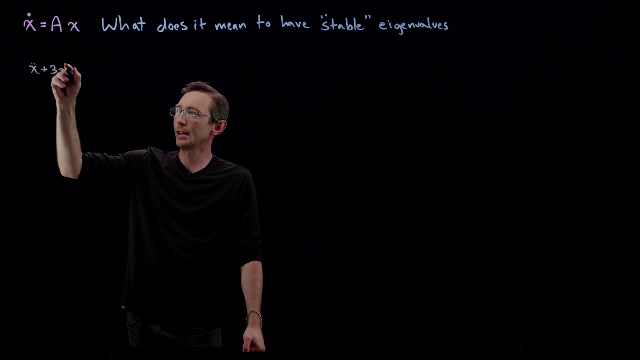 equation like x double dot plus three, x dot plus two x equals zero. we know that the solutions of this differential equation are things like you know: x of t equals. there's two fundamental solutions you can find from the characteristic polynomial And those two characteristic. 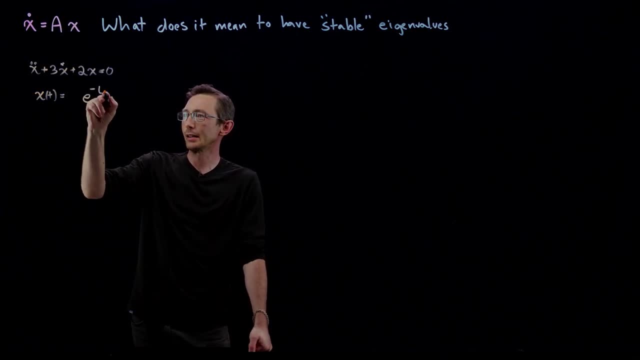 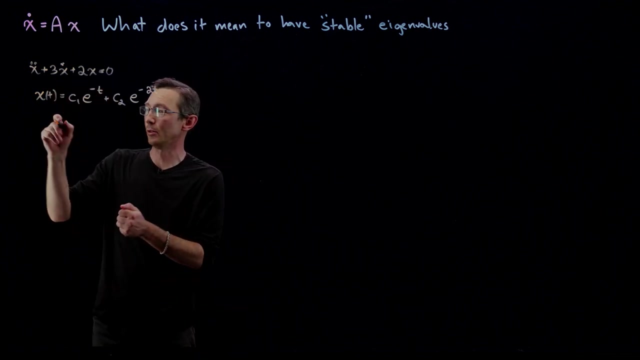 solutions are e to the minus t and e to the minus two t, And so any linear combination of these two solutions is all-in-one. So we know that the solutions of this differential equation are also a solution to this differential equation And we would say that this system is stable. 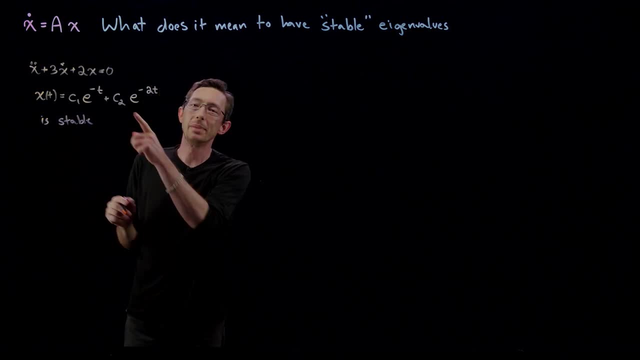 is stable because all of the fundamental solutions are stable, exponential. It's stable because all fundamental solutions, kind of- in this case there's only two fundamental solutions, but all the fundamental solutions- e to the minus t and e to the minus two t- are in fact stable. And literally what that means is, if I plot these functions as functions of time, 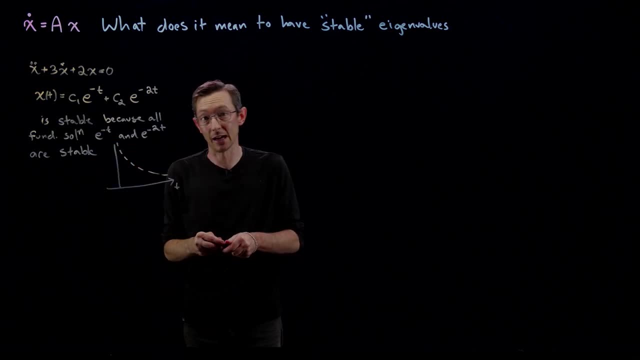 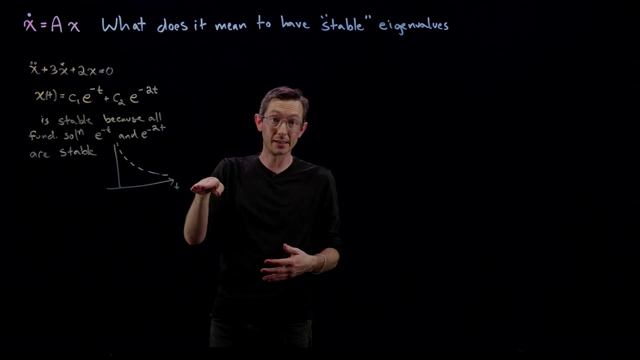 they are decaying exponentials. They decay to zero as time goes to infinity. So this is stable because the solution goes to zero, It remains bounded and, in fact, converges to zero asymptotically as t goes to infinity, as time goes to infinity. So that's what it means for this to be stable. 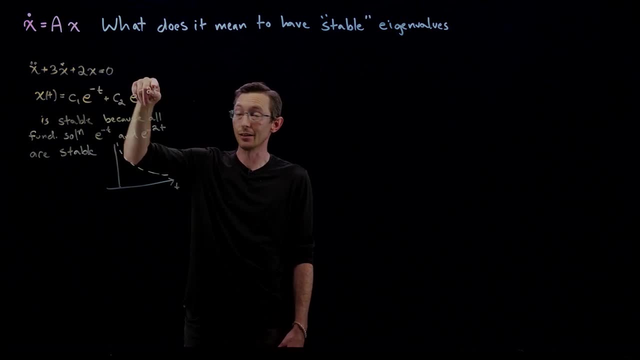 is that all of these powers of e to the minus t and e to the minus two t are stable, And so e to the minus two t are stable. They have negative, they're negative- real numbers. So e to the negative real number t is going to get, you know, arbitrarily small, as t goes to infinity. So how? 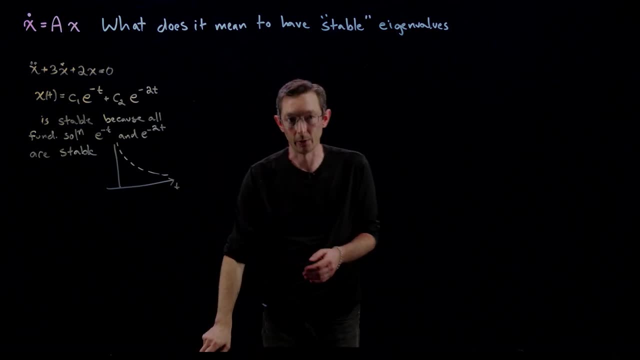 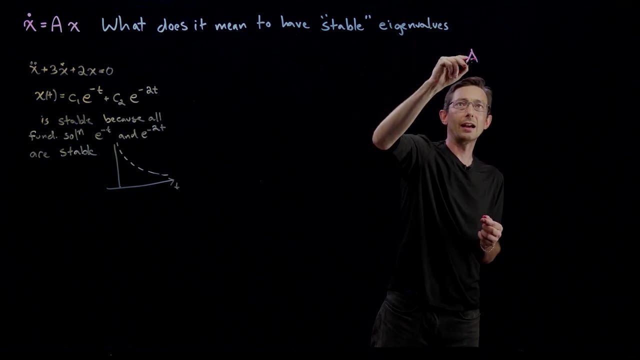 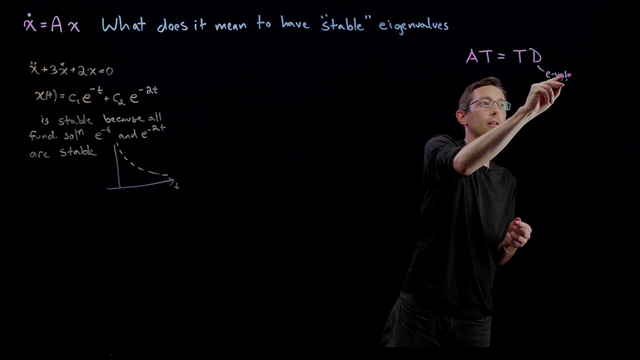 does that translate over to these matrix systems of differential equations? Well, we know, in this matrix system we're going to be talking about things like eigenvalues and eigenvectors. So we have a times t equals t times d, where these are my eigenvalues and these are my 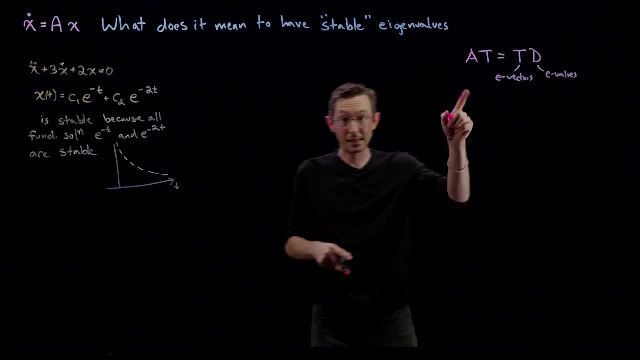 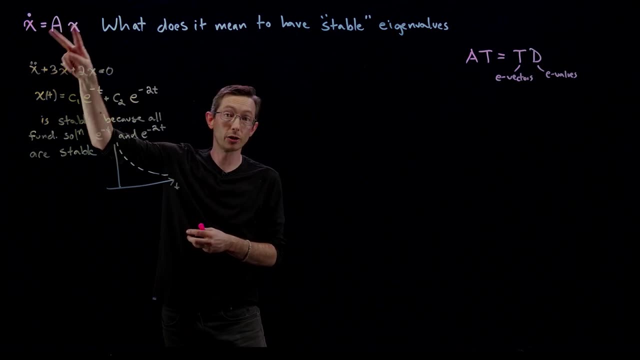 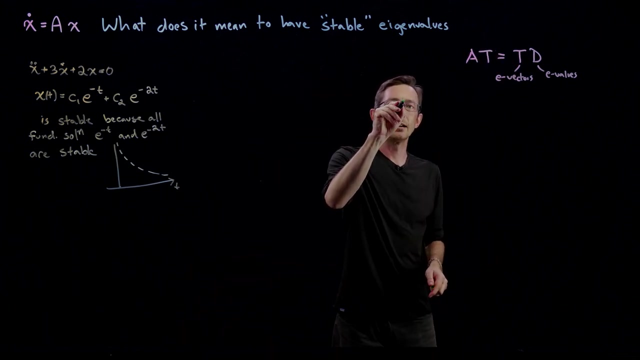 eigenvectors And specifically, what this eigendecomposition allows me to do is it allows me to write the solution of this differential equation in terms of these t's and d's in the following way. So we can write that x of t- the solution of my system at time- t is equal to. 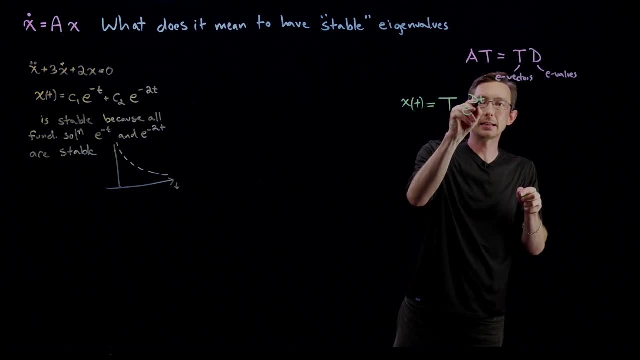 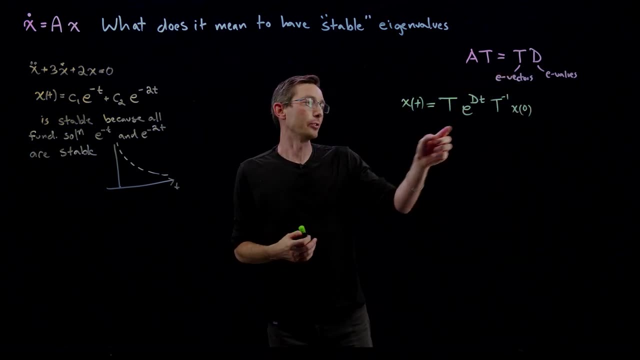 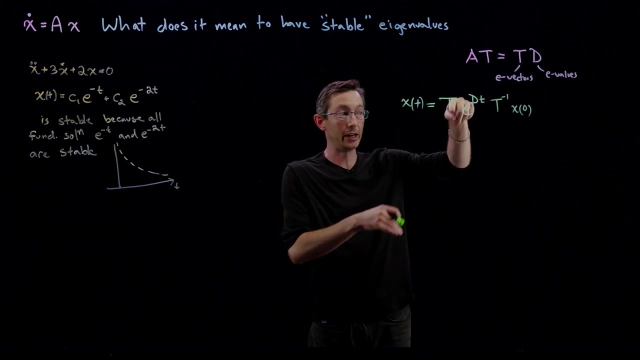 t times e to this diagonal matrix, d times t inverse times x naught And all of the action here. the only term that depends on time here is this: e to the diagonal matrix dt. Everything else is just a linear combination of the terms in this diagonal matrix. So I'm going to zoom in on this for a minute. We're going to 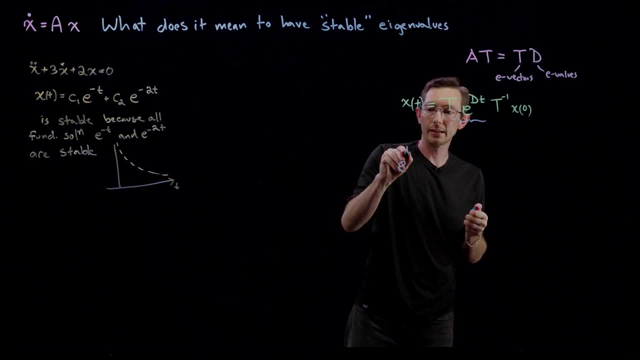 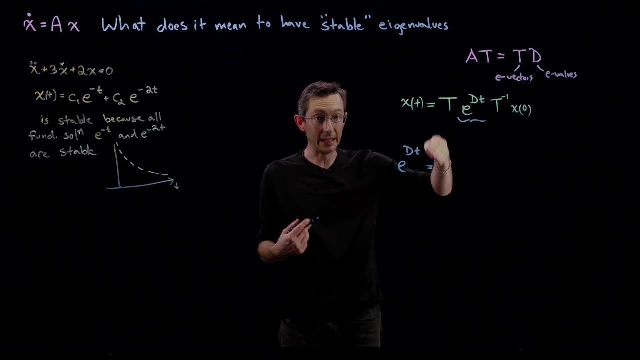 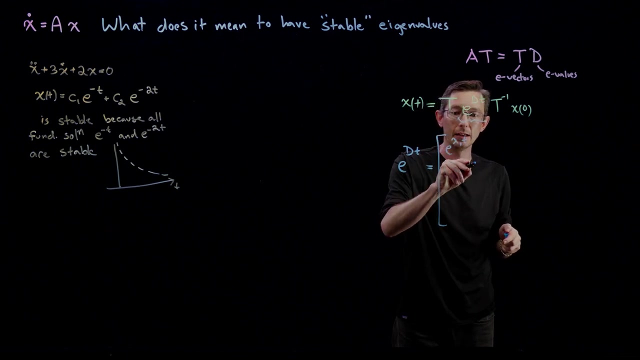 zoom in on this: e to the diagonal t. So e to the diagonal matrix t is a matrix, a diagonal matrix of e to the diagonal matrix dt, all of my eigenvalues of my matrix. So this is like e to my first eigenvalue, t, e to my second. 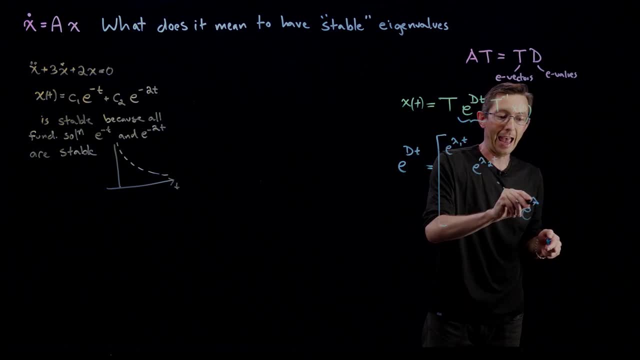 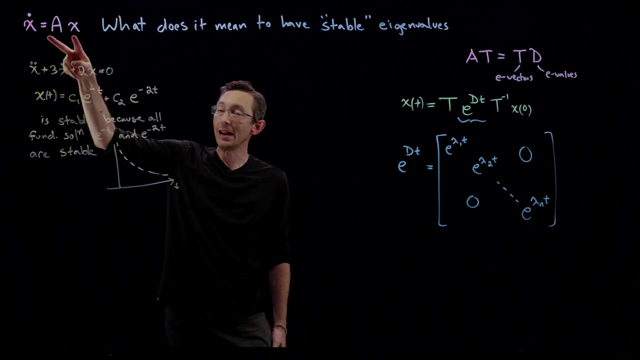 eigenvalue t, dot, dot, dot, dot, e to my nth eigenvalue, t, assuming that I have an n by n, square, a matrix and everything else is zero. And so here's what I mean: for an eigenvalue to be stable For this matrix system of equations- x, dot equals ax- to be stable. what it means is that: 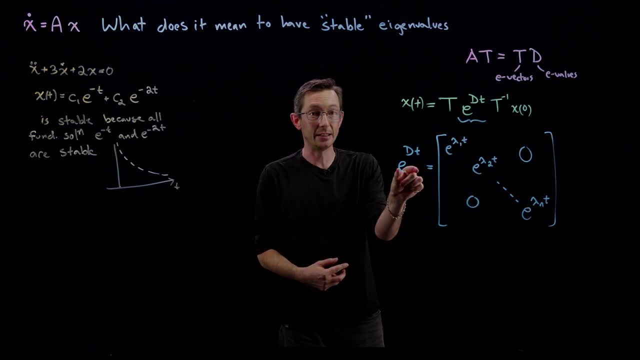 every single term in this diagonal matrix e to the dt, every single term here has to be stable. All of these have to be bounded, remain bounded and decay to zero as t goes to infinity. for this to be a stable system- Because I'm going to be taking these combinations, this t matrix and this- 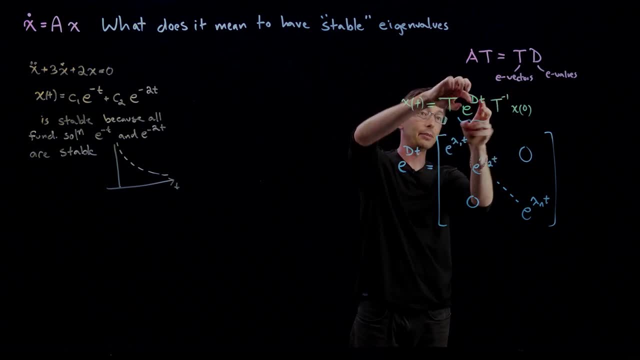 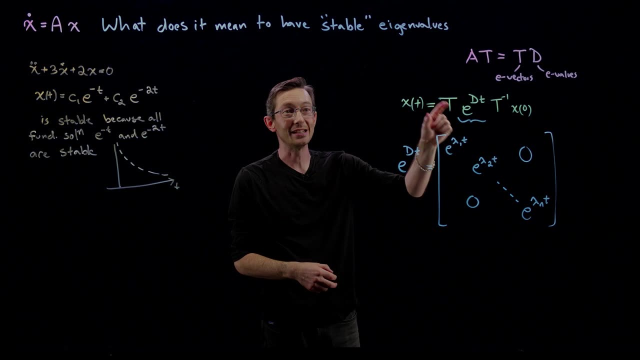 t inverse. these are inverses, convertible matrices. So I'm taking a combination of all of these e to the lambda t's and folding them up to build x of t, And so if even a single one of these is unstable, then my system is: 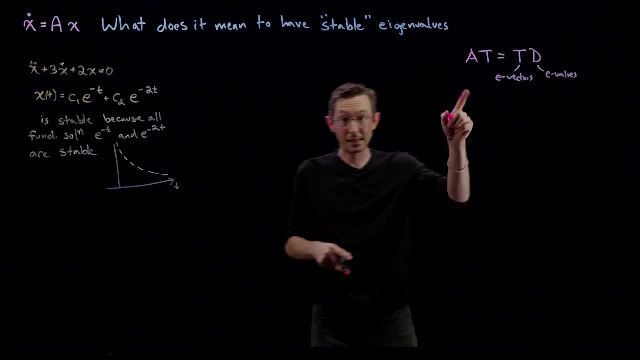 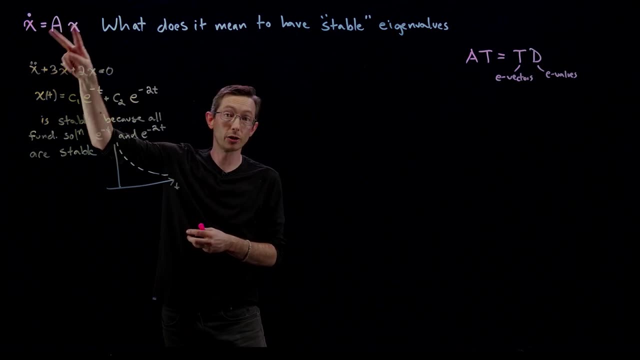 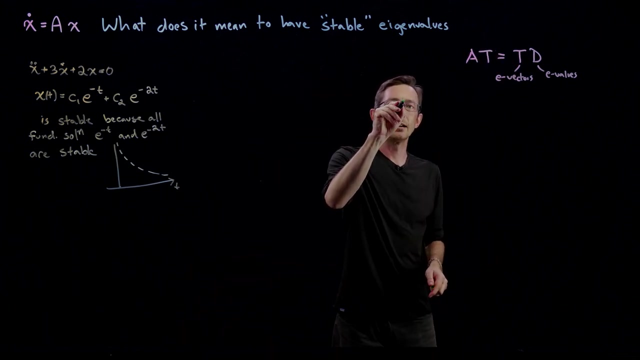 eigenvectors And specifically, what this eigendecomposition allows me to do is it allows me to write the solution of this differential equation in terms of these t's and d's in the following way. So we can write that x of t- the solution of my system at time- t is equal to. 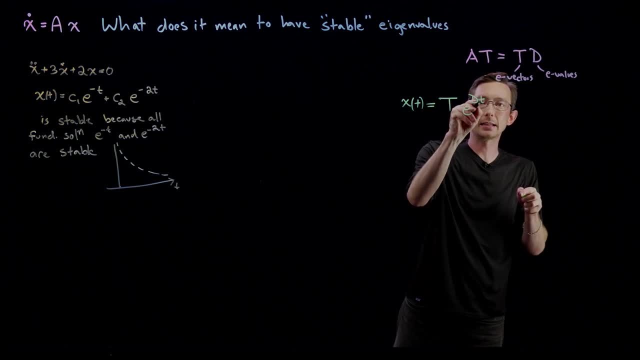 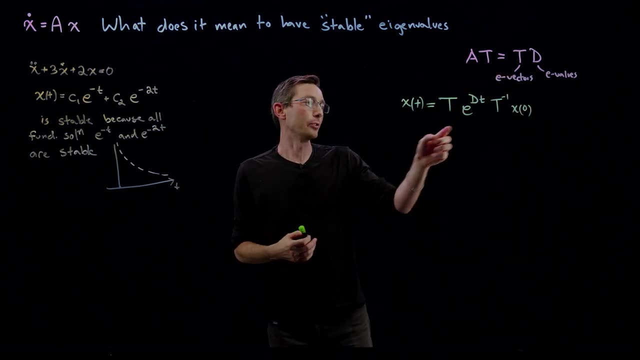 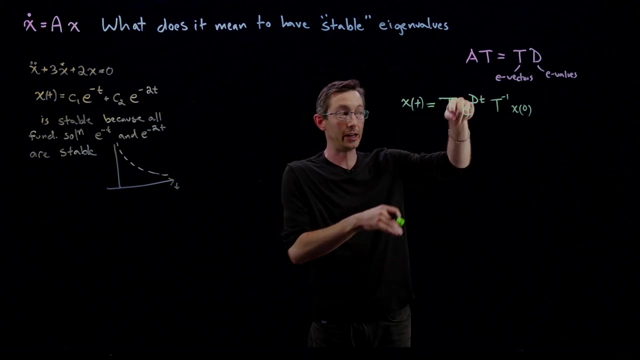 t times e to this diagonal matrix, d times t, inverse, times x-naught And all of the action here. the only term that depends on time here is this: e to the diagonal matrix dt. Everything else is just a linear combination of the terms in this diagonal matrix. So I'm going to zoom in on this for a minute. we're going to 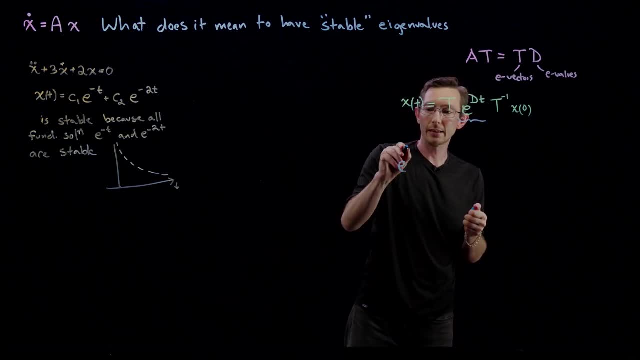 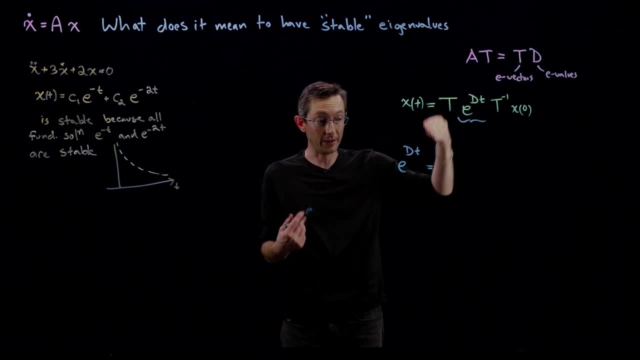 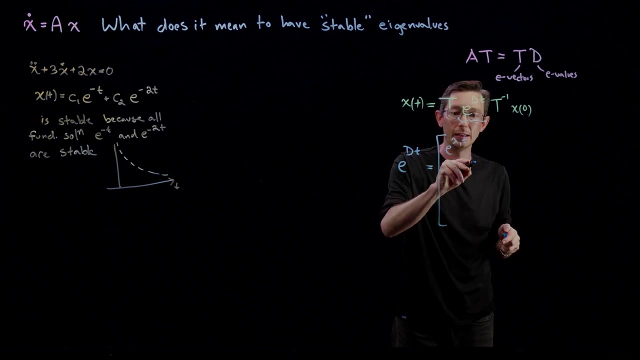 zoom in on this: e to the diagonal t. So e to the diagonal matrix t is a matrix, a diagonal matrix of e to the diagonal matrix dt, all of my eigenvalues of my matrix. So this is like e to my first eigenvalue, t, e to my second. 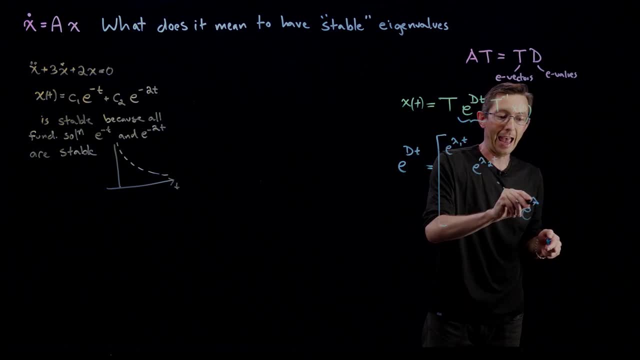 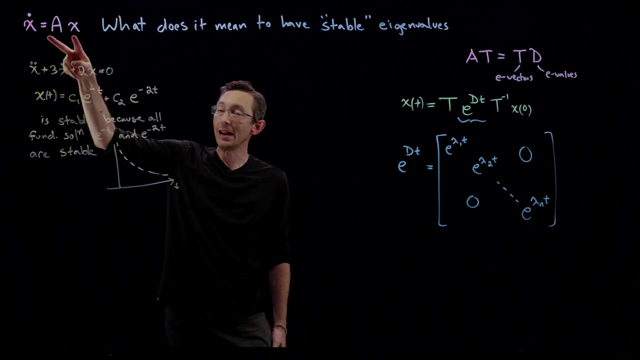 eigenvalue t, dot, dot, dot, dot e to my nth eigenvalue, t, assuming that I have an n by n, square, a matrix and everything else is zero. And so here's what I mean for an eigenvalue to be stable For this matrix system of equations- x- dot equals a x- to be stable. what it means is that: 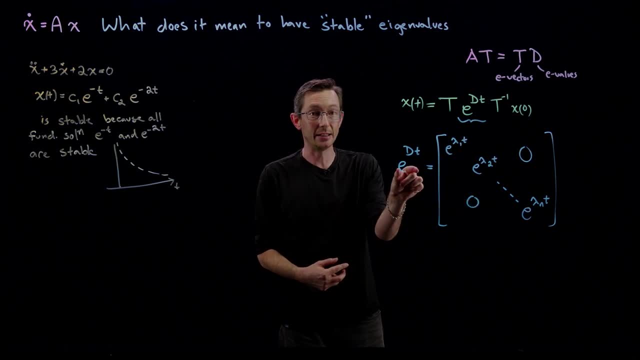 every single term in this diagonal matrix e to the dt, every single term here has to be stable. All of these have to be bounded, remain bounded and decay to zero as t goes to infinity. for this to be a stable system- Because I'm going to be taking these combinations, this t matrix and 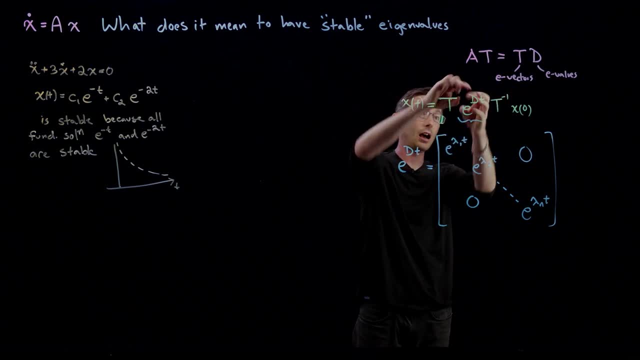 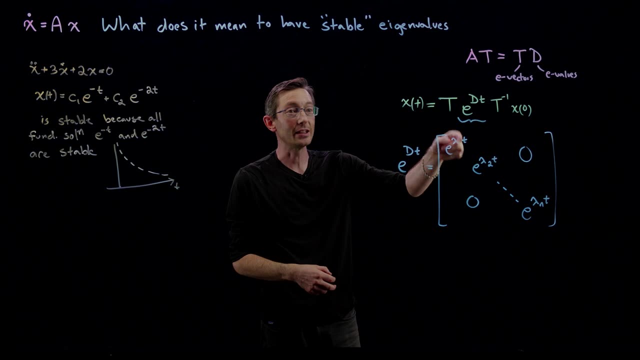 t inverse. these are inverses, convertible matrices. So I'm taking a combination of all of these e to the lambda t's and folding them up to build x of t, And so if even a single one of these is unstable, then my system is: 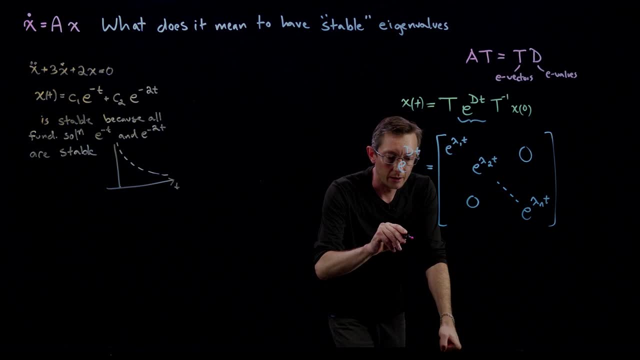 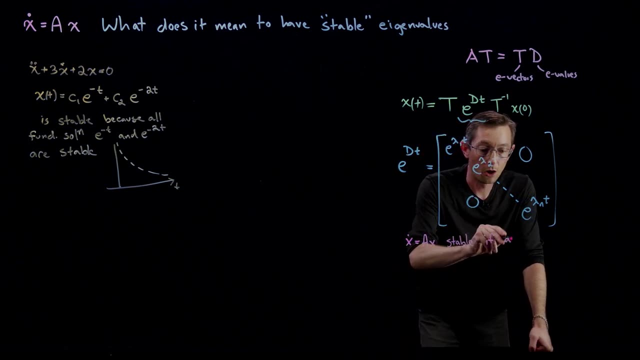 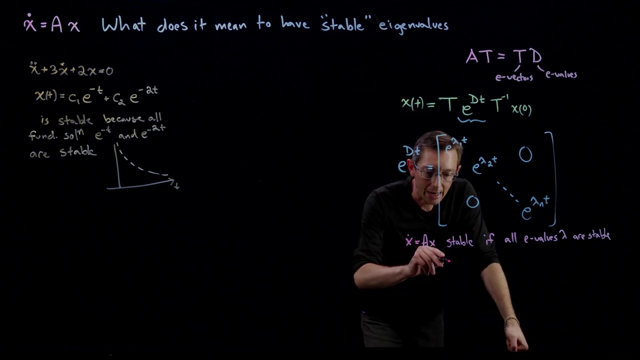 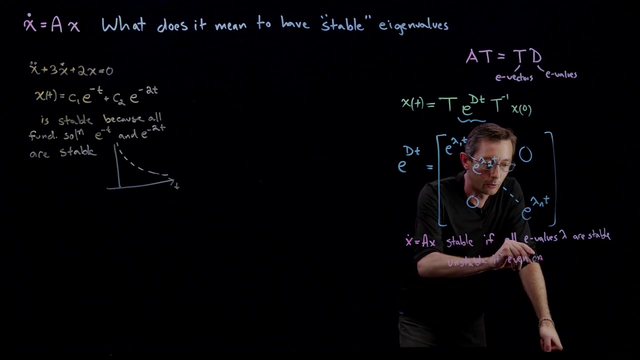 unstable. So let me write that out. So x dot equals a. x is stable if all eigenvalues- lambda- are stable, And I'm going to say I'll tell you what that means in a minute. it means they all have negative real part, OK, And it's unstable if even one, or at least one, if even a single. 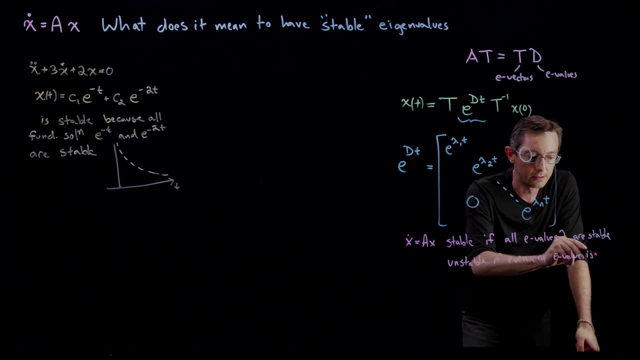 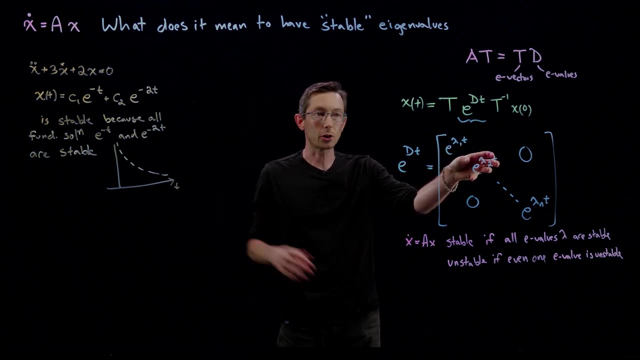 eigenvalue is unstable. OK, And now does that make sense? Because if even one of these terms blows up, then my system is unstable. So I'm going to take a combination of all of these up to infinity, and all of the other ones are stable. let's say: you know all of 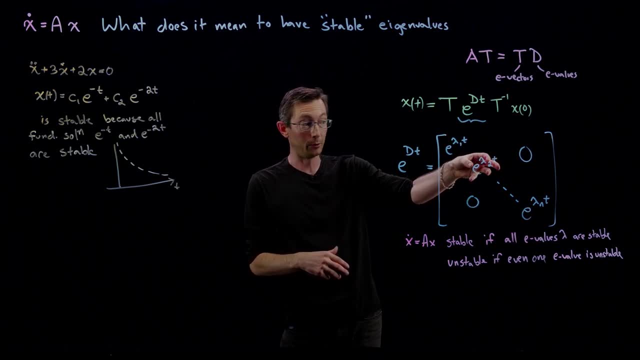 them are stable except for this one, and this one blows up to infinity because it's unstable. when I take this linear combination of all of these terms and I fold this up, X of T is still gonna blow up to infinity because this term is gonna dominate everything else. and it's gonna blow up to infinity so even one. 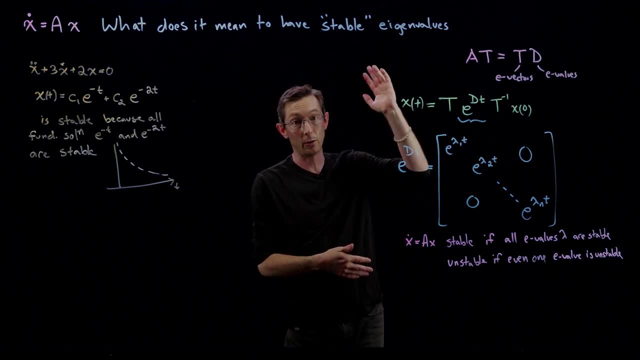 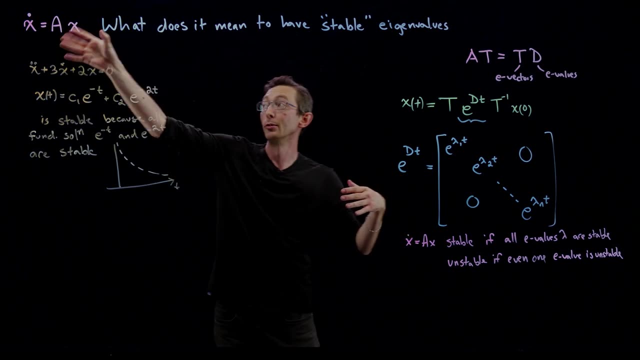 bad apple. one unstable eigenvalue is gonna blow up my whole solution and my systems unstable. so all of the eigenvalues have to, all of these behaviors have to be stable for my global system to be stable. okay, so now I'm gonna show you what it means for an eigenvalue to be stable here. this was. 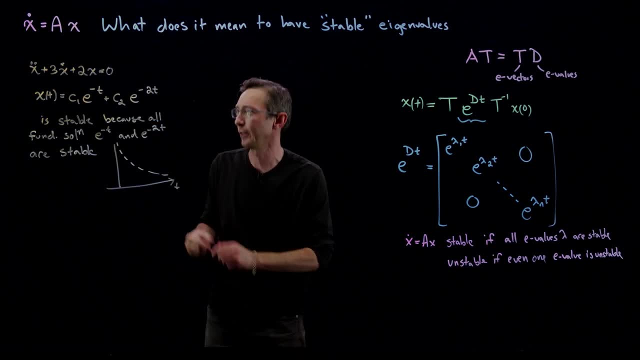 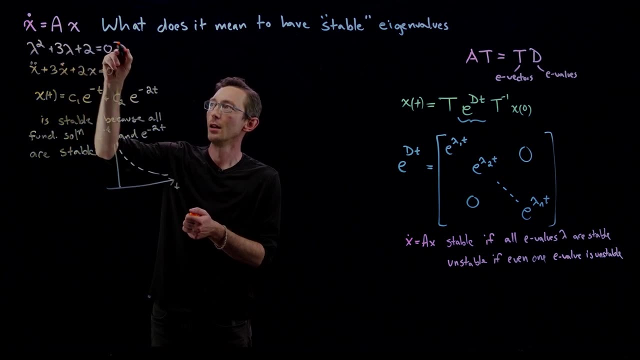 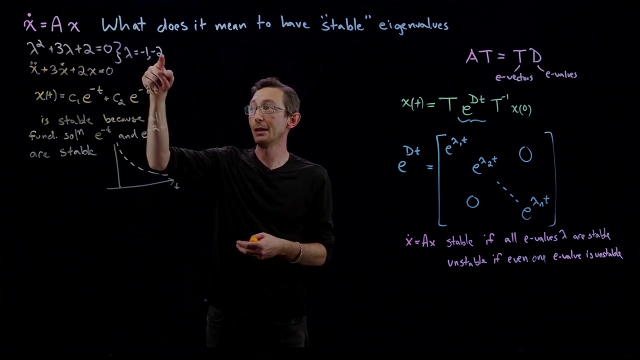 pretty simple, because these are real valued lambdas. if we did our characteristic equation lambda squared plus 3, lambda plus 2 equals 0. we find that lambda equals minus 1 and minus 2. so these are both real valued lambdas and they're stable because they're negative. okay, either the negative power T. 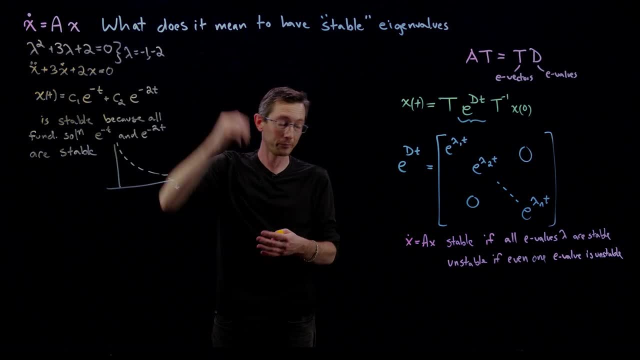 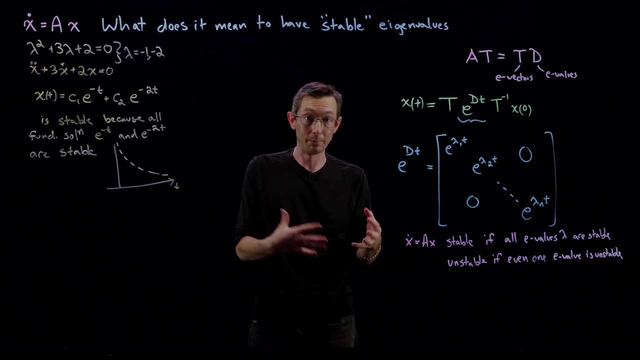 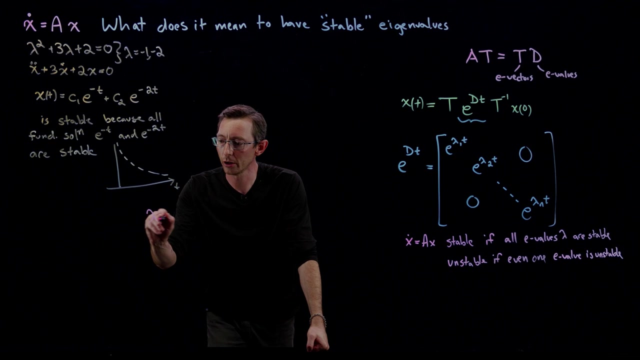 is stable, e to the positive power, T is unstable. but here, when we're talking about a generic matrix system, these eigenvalues can actually come in complex conjugate pairs, so it's a little more subtle than that. okay, so my lambda, my lambdas could come in complex conjugate pairs: A plus IB and. 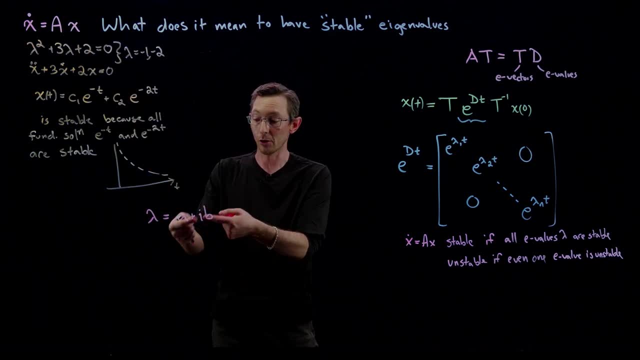 of course, if I had an A plus IB for a real valued matrix, I would also have to have another eigenvalue, A minus IB. but let's just say, now that we have an eigenvalue A minus IB and it's now a real value matrix, I would also have to have another eigenvalue, A minus IB. but let's just. 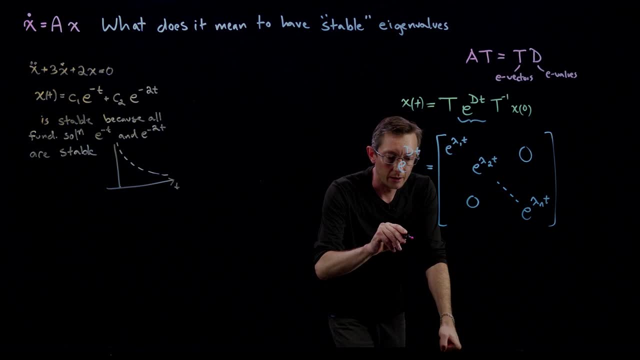 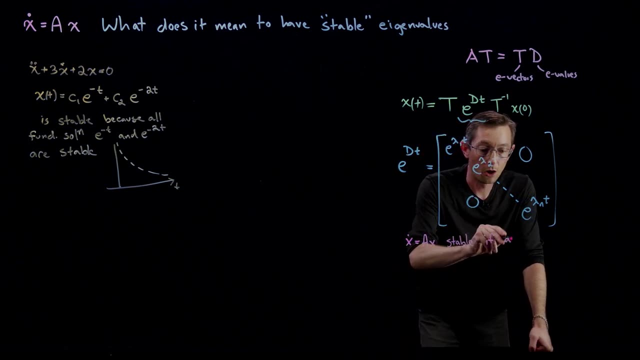 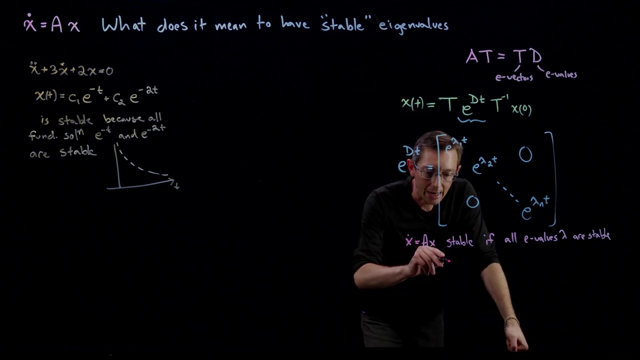 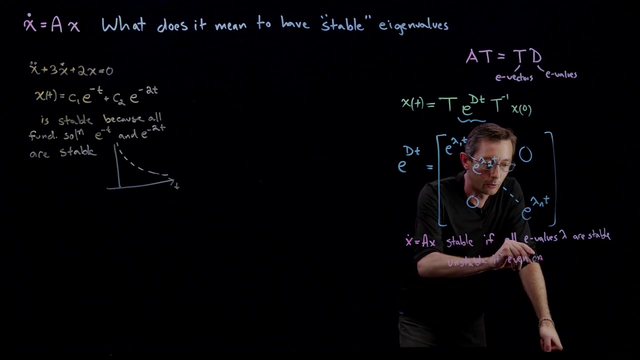 unstable. So let me write that out. So x dot equals a. x is stable if all eigenvalues- lambda- are stable, And I'm going to say I'll tell you what that means in a minute. it means they all have negative real part, okay, And it's unstable if even one, or at least one, if even a single. 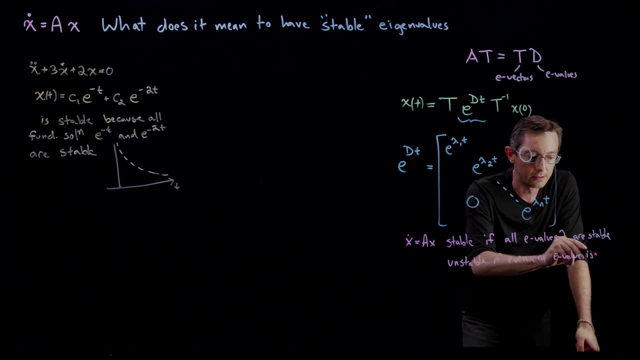 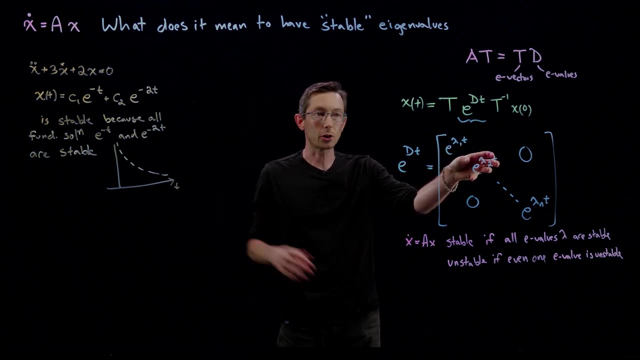 eigenvalue is unstable. okay, And now does that make sense? Because if even one of these terms blows up, then my system is unstable. So if even one of these terms blows up, then my system is up to infinity and all of the other ones are stable. let's say: you know all of 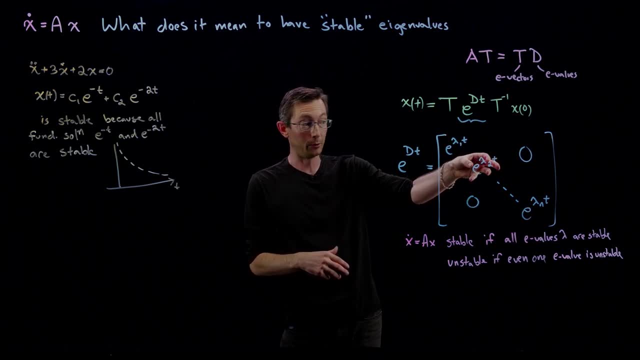 them are stable except for this one, and this one blows up to infinity because it's unstable. when I take this linear combination of all of these terms and I fold this up, X of T is still gonna blow up to infinity because this term is gonna dominate everything else. and it's gonna blow up to infinity so even one. 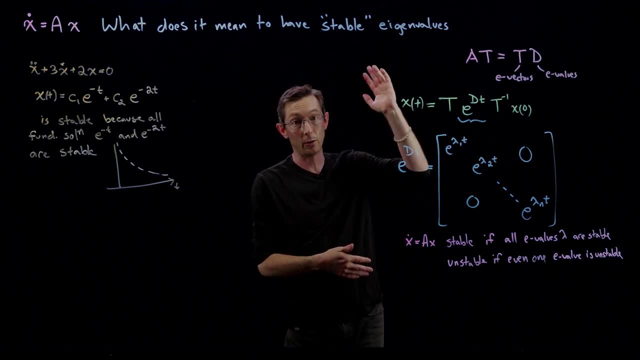 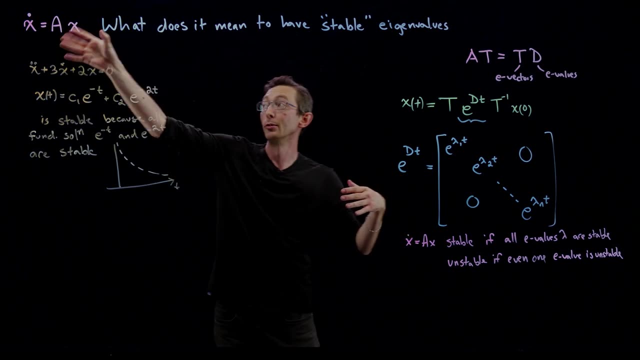 bad apple. one unstable eigenvalue is gonna blow up my whole solution and my systems unstable. so all of the eigenvalues have to, all of these behaviors have to be stable for my global system to be stable. okay, so now I'm gonna show you what it means for an eigenvalue to be stable here. this was. 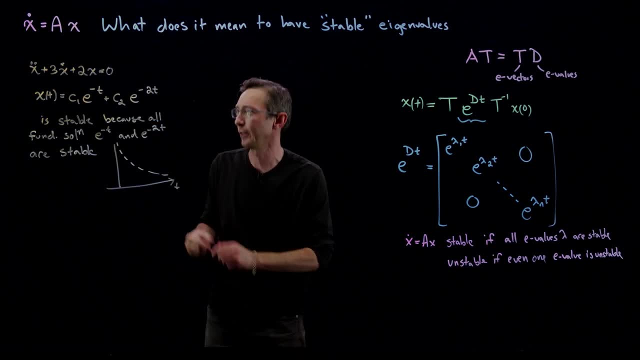 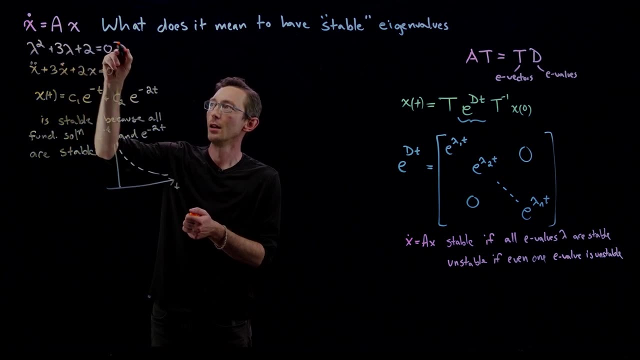 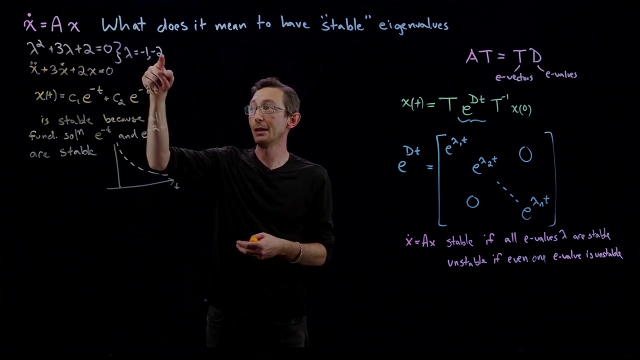 pretty simple, because these are real valued lambdas. if we did our characteristic equation lambda squared plus 3, lambda plus 2 equals 0. we find that lambda equals minus 1 and minus 2. so these are both real valued lambdas and they're stable because they're negative. okay, either the negative power T. 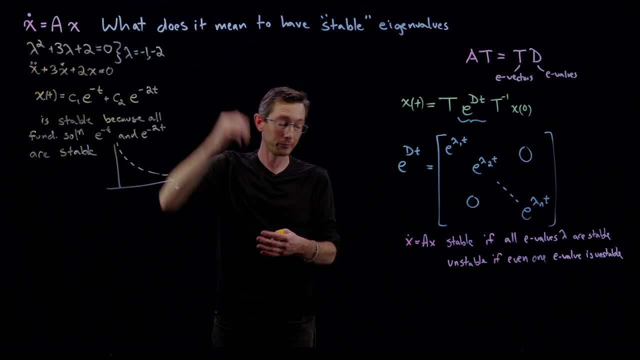 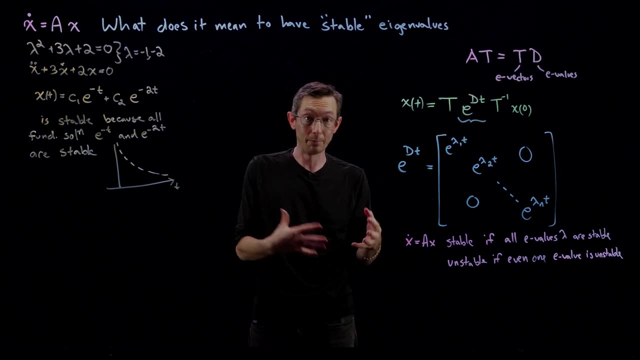 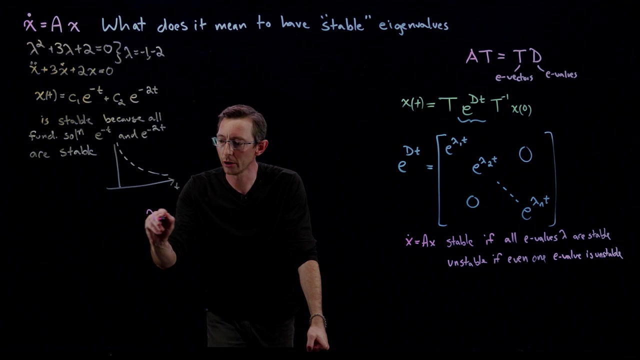 is stable either. the positive power T, is unstable. but here, when we're talking about a generic matrix system, these eigenvalues can actually come in complex conjugate pairs, so it's a little more subtle than that. okay, so my lambda, my lambdas could come in complex conjugate pairs: a plus i, B. and, of course, if I had, 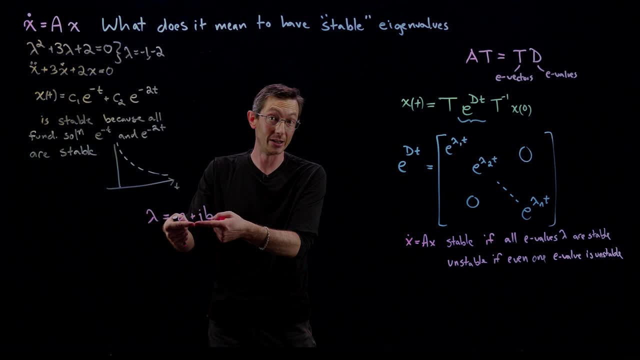 an a plus i B for a real valued matrix, I would also have to have another eigen value: a minus i B. but let's just say, if I had a plus i B for a real valued matrix, I would also have to have another agen value: a minus i B. but let's just 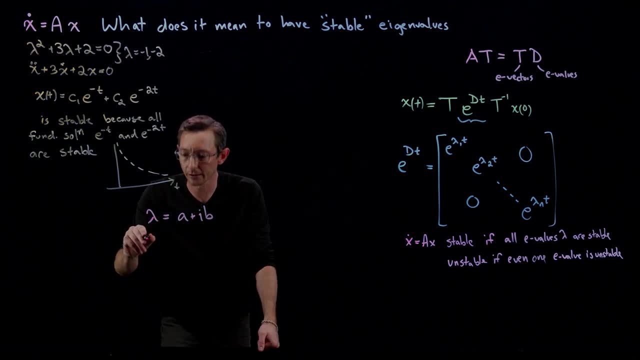 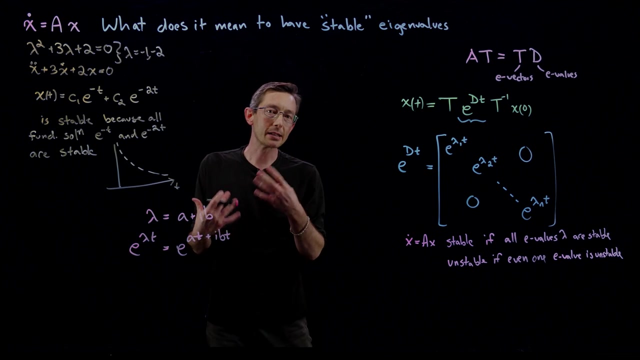 just look at this one for now. okay, And so if I take e to the lambda t, that equals e to the a plus, let's say, at plus ibt, because I can multiply both of these by t And because of. 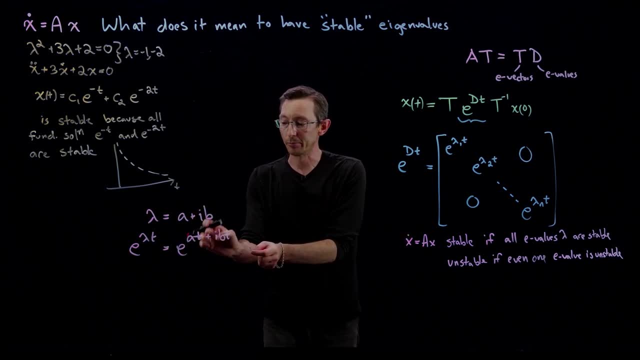 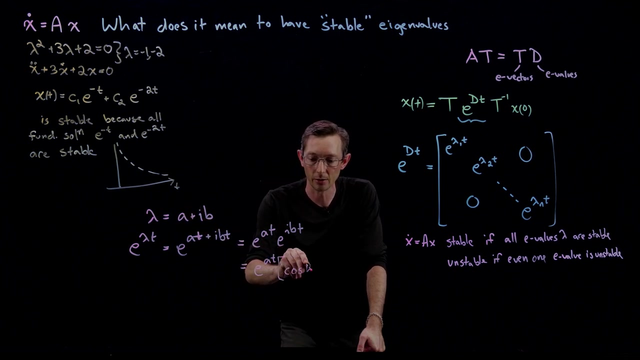 the property of exponentials, e to the at plus ibt, equals e to the at times, e to the ibt. This is really, really useful. And now, finally, I'm going to use Euler's formula to expand this out, And we're going to see that this equals e to the real part at times, something like cosine bt. 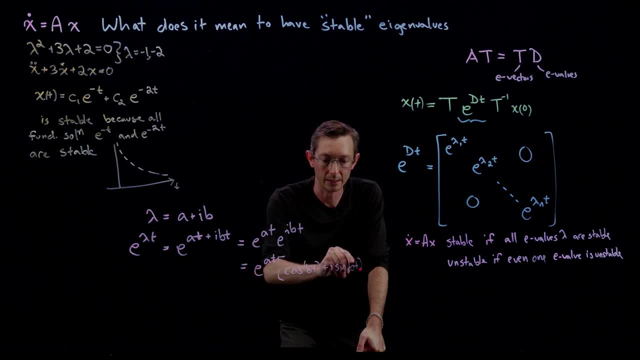 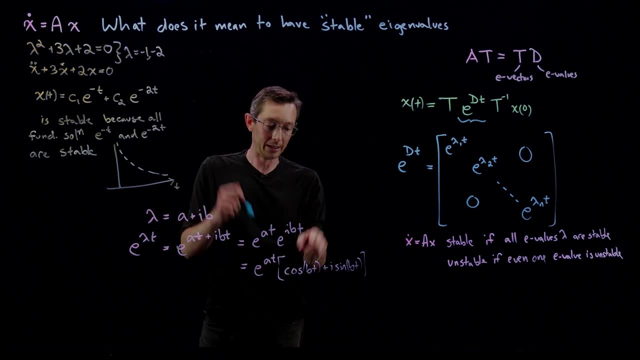 plus i sine bt. And what I want to point out here is that this number has kind of unit length. That's a complex number, You know it's got a real and an imaginary part, But this has a unit length And it's a real and an imaginary part, And it's a real and an imaginary part And it's. 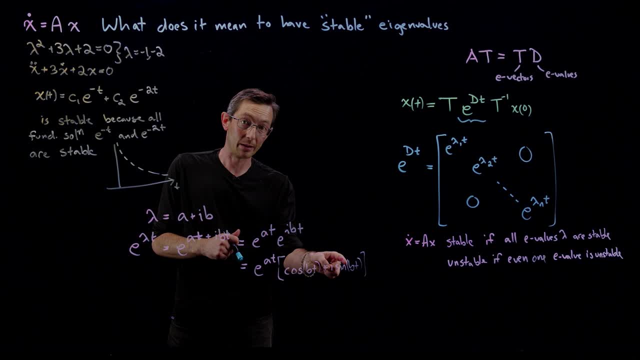 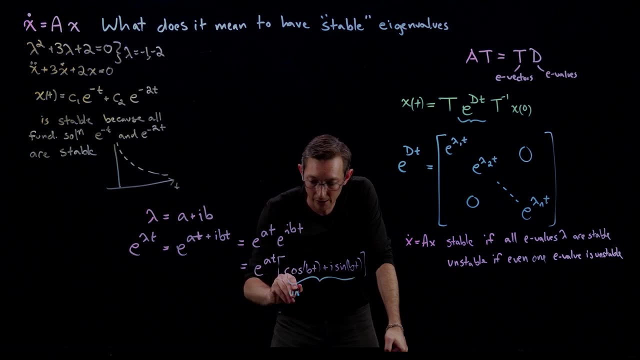 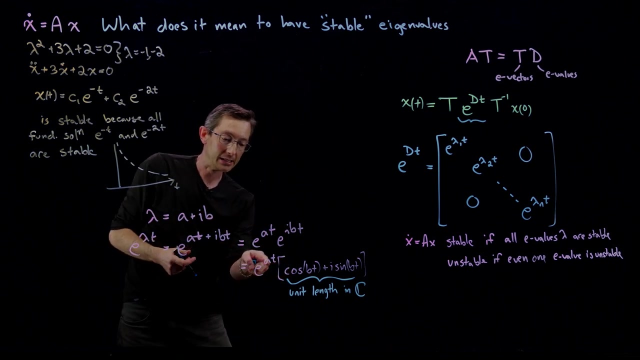 the real part squared plus the imaginary part squared is cosine. squared plus sine squared equals one. this has unit length in the complex plane. this is like unit length or size or norm. sometimes we call it norm, unit norm in the complex plane, and the only thing that can make this solution blow up or decay is this e to. 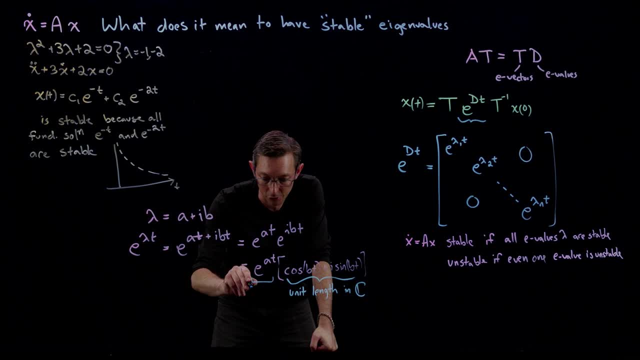 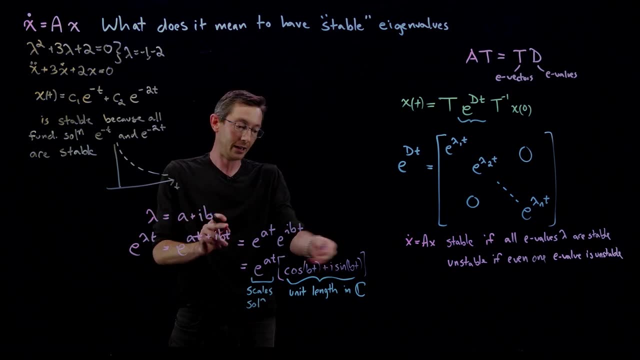 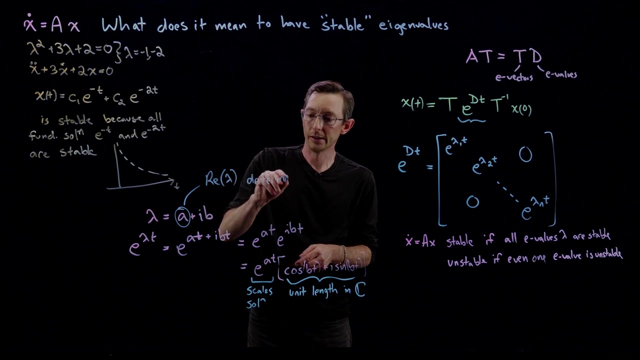 the a, t. so this scales the solution, this scales the solution, this kind of oscillating solution. if I have a plus IB, then I get some oscillation at frequency B. and this real part here, this real part of lambda, so the real part of lambda is what determines stability, determines stability. 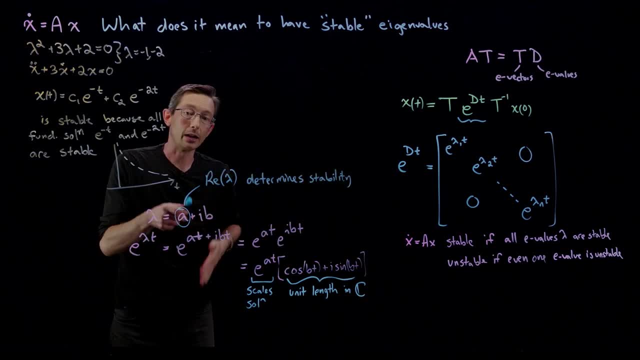 because if this actually alpha, if this a here is positive, then this oscillating part is multiplied by e to the positive a, t. that's going to blow up to infinity. that's going to be unstable. so if a is positive, my system is unstable. if a is negative, this is e. 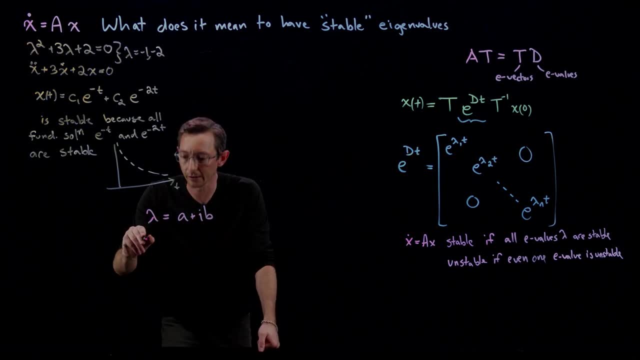 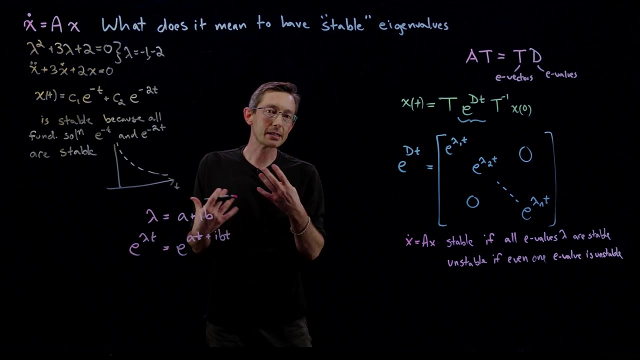 look at this one for now. okay, and so if I take e to the lambda t, that equals e to the a plus. let's say a t plus i b t, because I can multiply both of these by t and because of the property of exponentials, e to the a t plus i b t. 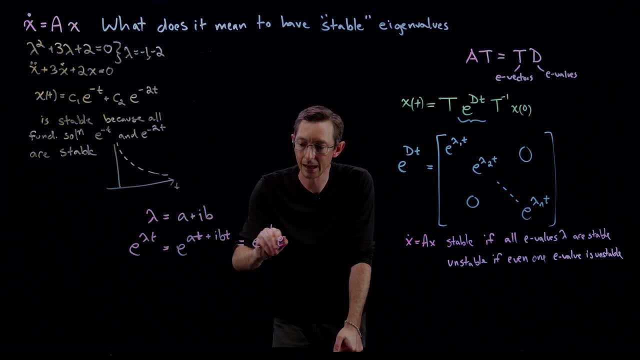 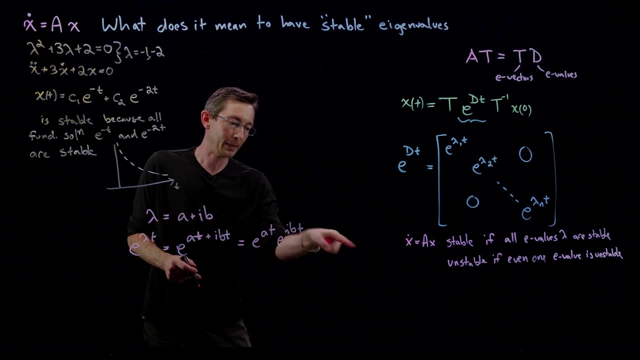 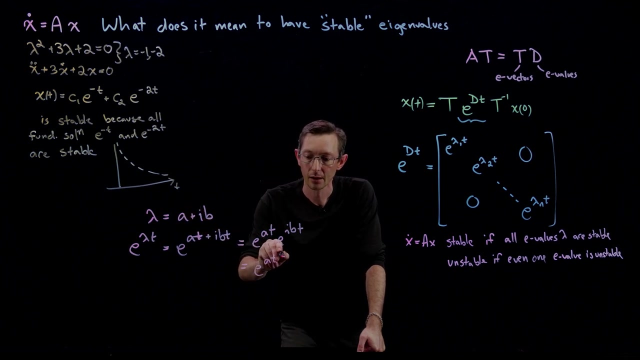 equals e to the a t times e to the i b t. this is: this is really really useful. and now, finally, I'm going to use Euler's formula to expand this out, and we're going to see that this equals e to the- the real part a t times something like. 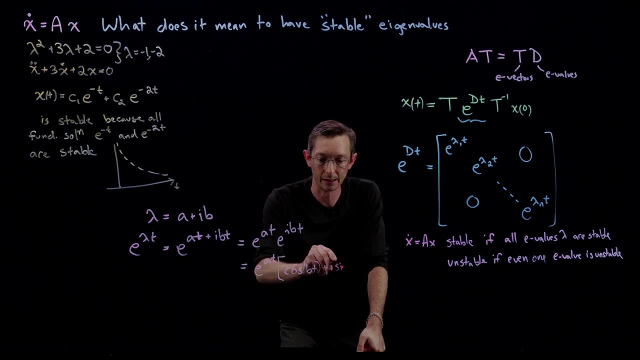 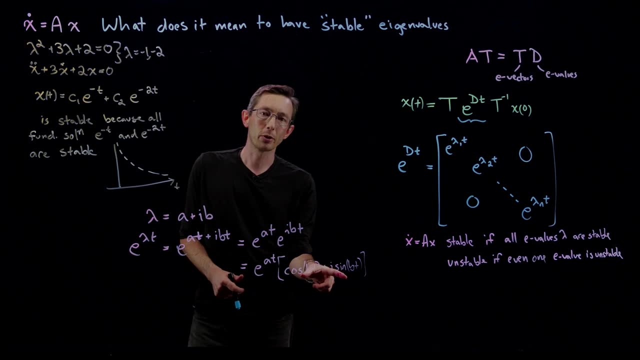 cosine b t plus i sine b t. and what I want to point out here is that this number has kind of unit length. that's a complex number, you know it's got a real and an imaginary part, but this has a unit length, the real part squared plus the. 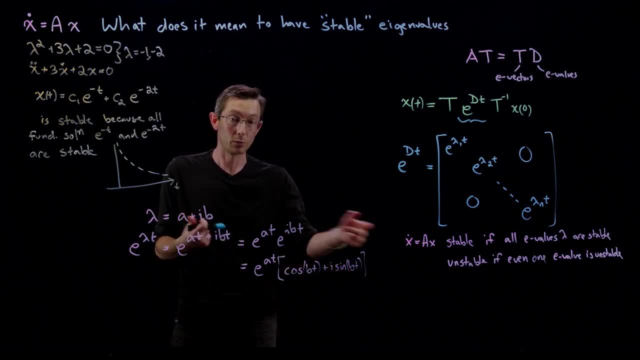 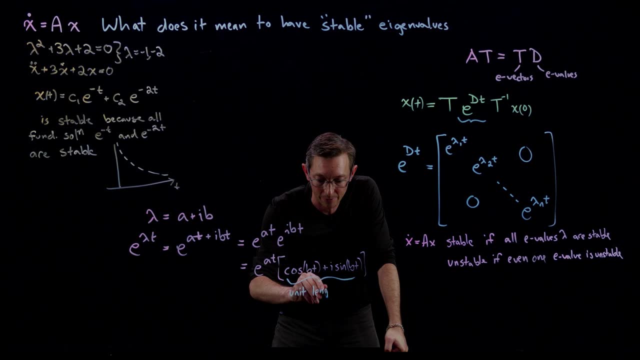 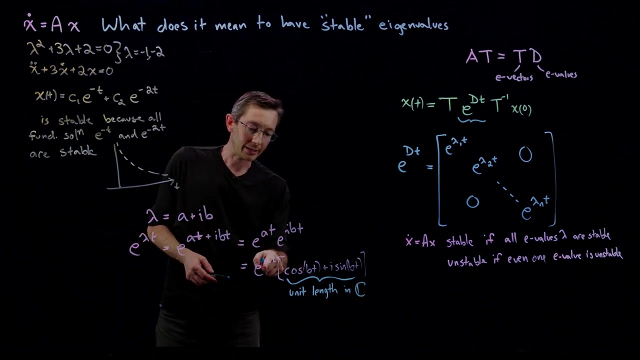 imaginary part. squared is cosine squared plus sine. squared equals one. this has unit length in the complex plane. this is like unit length or size or norm. sometimes we call it norm, unit norm in the complex plane, and the only thing that can make this solution blow up or decay. 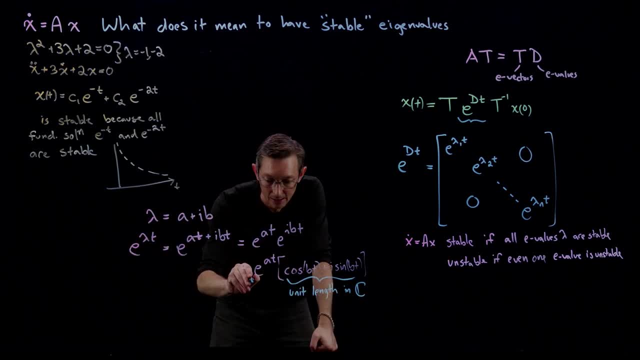 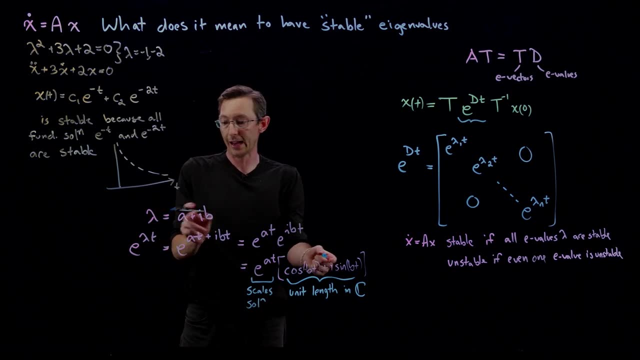 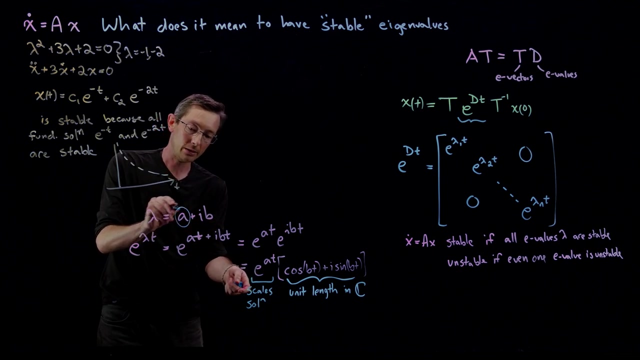 is this: e to the a, t, so this scales the solution. this scales the solution, this kind of oscillating solution. if I have a plus IB, then I get some oscillation at frequency B, and this real part here, this real part of lambda, so the real part of 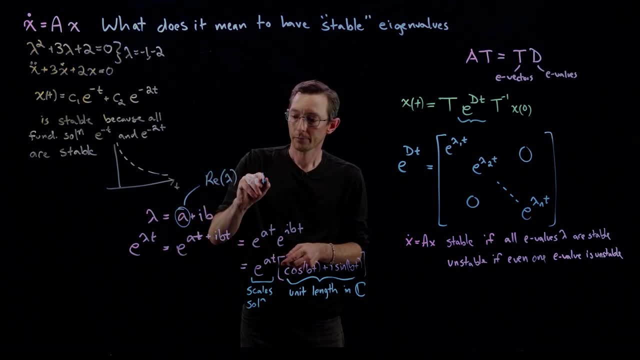 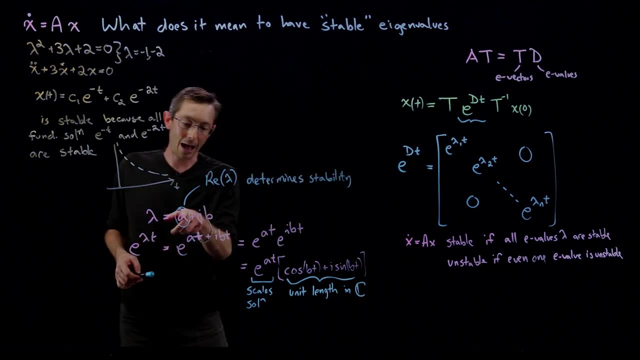 lambda is what determines stability. determines stability because if this alpha, if this a here is positive, then this oscillating part is multiplied by e to the positive a, t. that's going to blow up to infinity. that's going to be unstable. so if a is positive, my system is unstable. if a is. 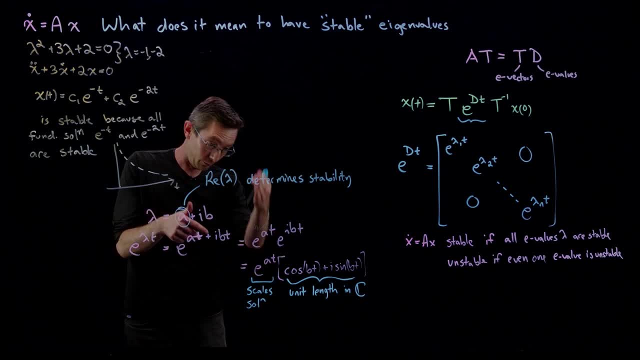 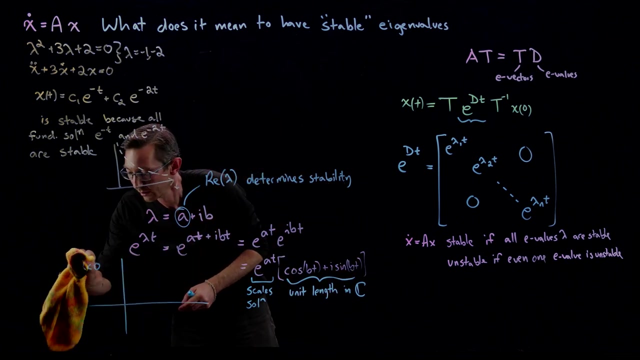 negative. this is e- to the minus number T, it will be stable and decay to zero. so in this case, here that I've drawn, if I have like a less than zero, this alpha- sorry, it's not alpha, it's a- if a is less than zero. maybe really careful here not to confuse. 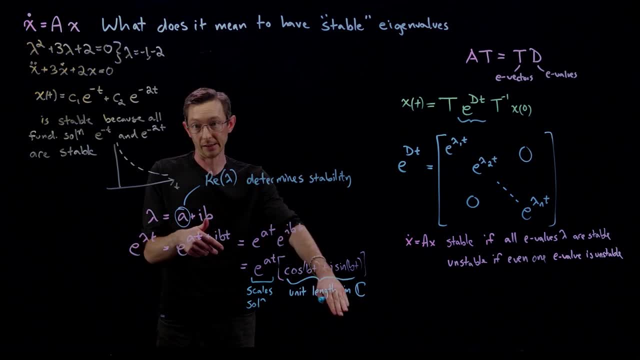 to the minus number t, it will be stable and decay to zero. so in this case here that I've drawn, if I have like a less than zero, this alpha- sorry, it's not alpha, it's a- if a is less than zero, maybe really careful here not to confuse you with bad symbol writing. if 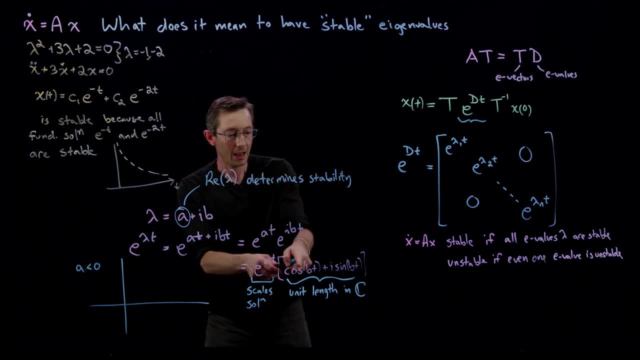 the real part of my eigenvalue is less than zero and I have some, you know, maybe I have some plus IB, so I have some oscillation. I'm going to get an oscillation multiplied by this decaying exponential envelope, so I'm going to have my solution look stable as time goes to infinity. okay, that's what I mean. 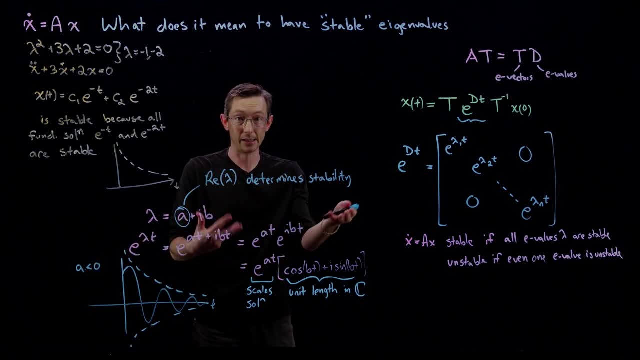 by a less than zero, because I don't want boost over this value. so if I can get my solution from it- and I'm going to get that- a less than zero. less than zero gives me a stable system And similarly- maybe I'll move this over a little- 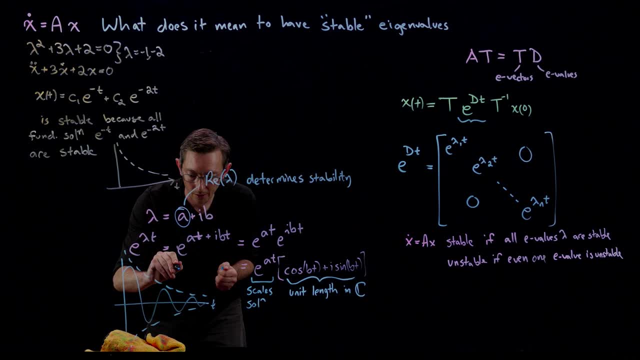 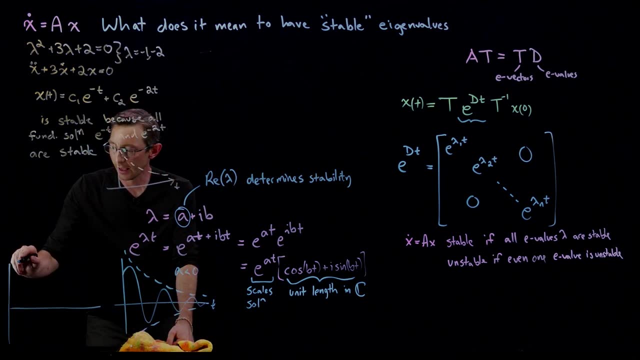 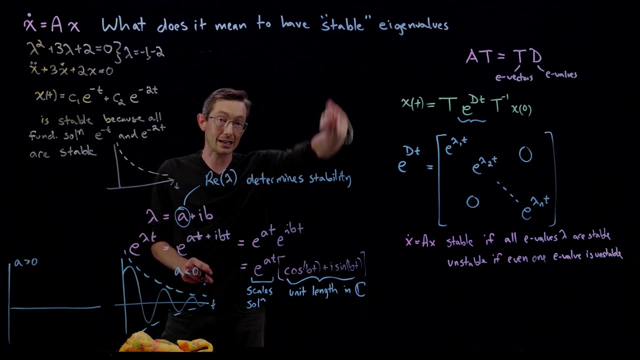 bit. So this is the a less than zero. If I look at the a greater than zero case, if I have the a greater than zero case, so the real part of my eigenvalue is greater than zero. now I'm multiplying this by a growing exponential envelope, So now my envelope is growing. 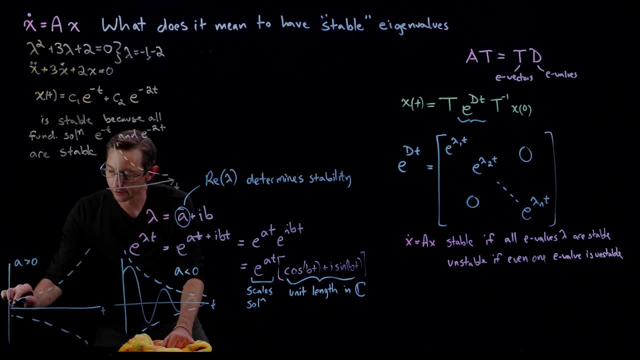 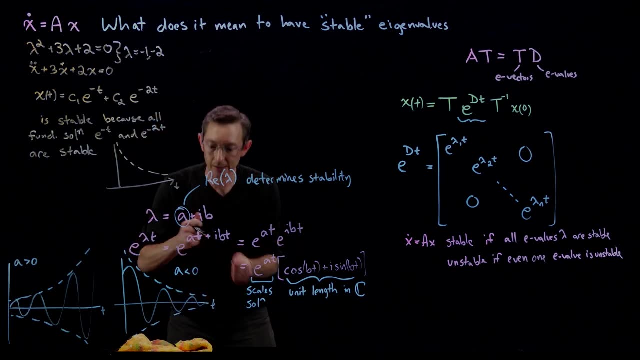 exponentially in time, And so now my oscillation is going to be growing in amplitude, and this would be an unstable system. So a less than zero is stable, A greater than zero: if my real part of my eigenvalue is greater than zero, then it's unstable, And if a equals zero. so I only have 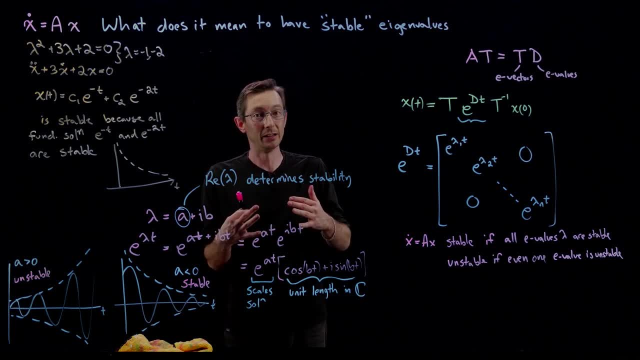 this oscillating part. we call that neutrally stable. It is bounded and it's not blowing up to infinity, but it's also neutral. It's not decaying to zero. It's just kind of sines and cosines and it's going to oscillate. 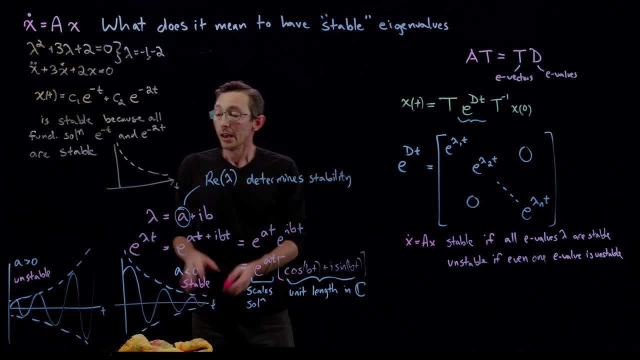 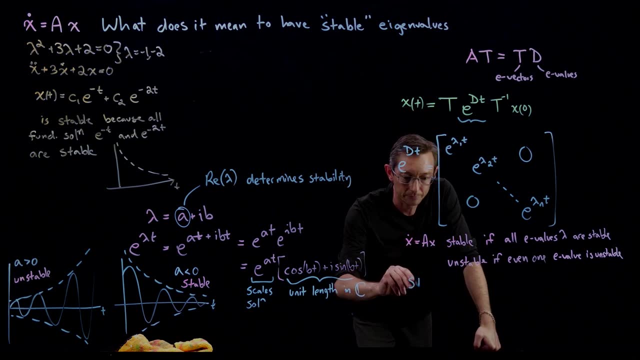 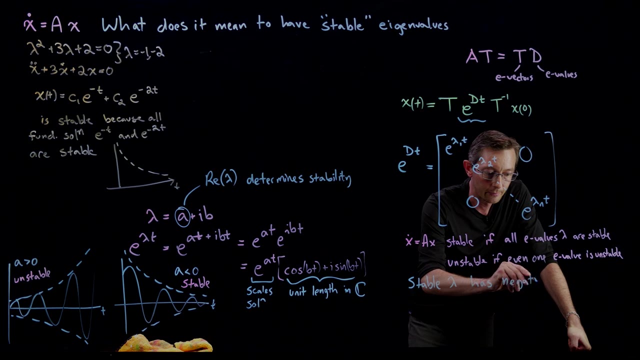 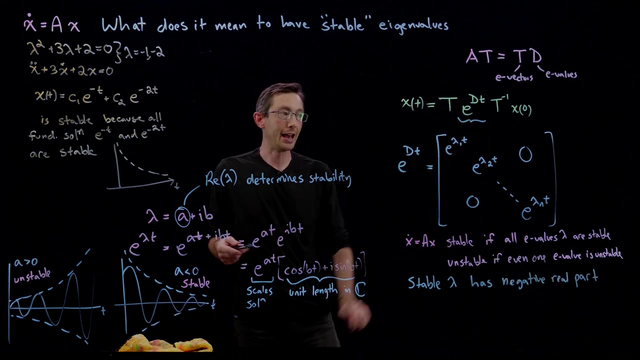 at the same amplitude forever if a equals zero. So this is super, duper important. And what I mean by stable here is a stable lambda has negative real part. The imaginary part has nothing to do with the stability of that eigenvalue, It just causes us. 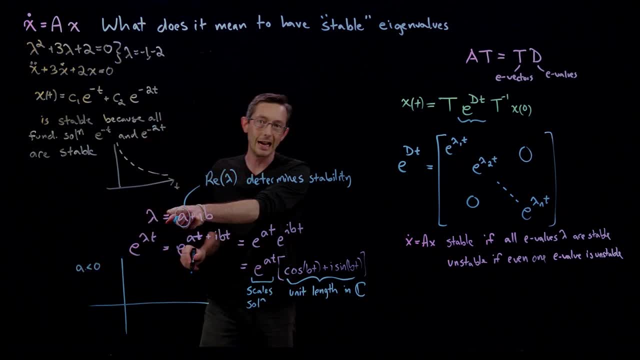 you with bad symbol writing. if the real part of my eigenvalue is less than zero- and i have some, you know, maybe i have some uh plus ib, so i have some oscillation. i'm going to get an oscillation multiplied by this decaying exponential envelope. so i'm going to have 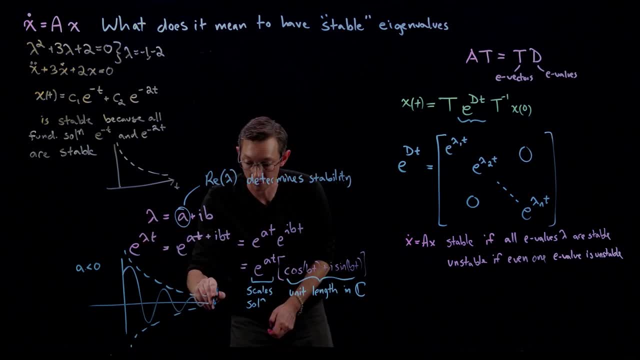 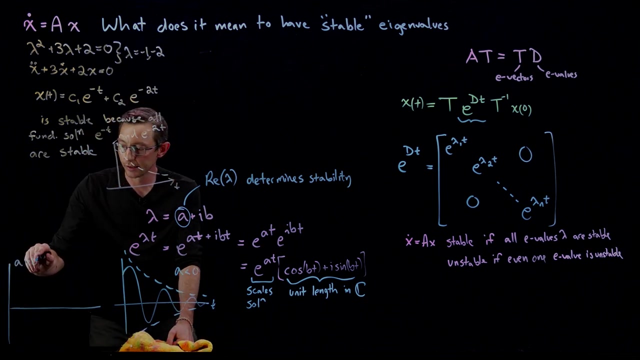 my solution: look stable as time goes to infinity. okay, that's what i mean by a less than zero- gives me a stable system and similarly- maybe i'll move this over a little bit. so this is the a less than zero. if i look at the a greater than zero case, if i have the- uh, a greater than zero. 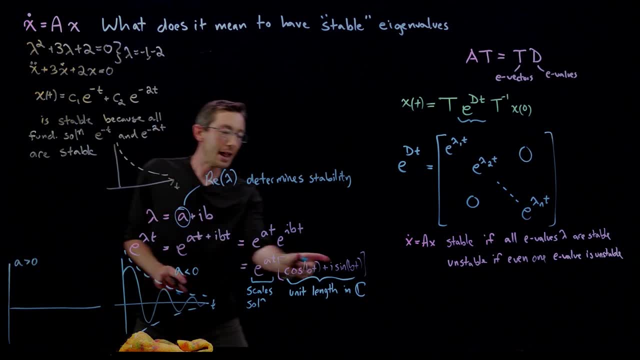 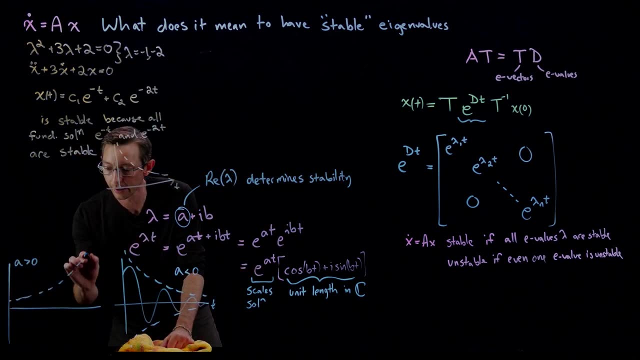 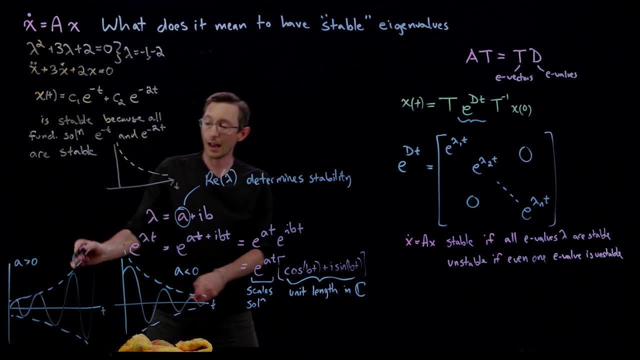 case. so the real part of my eigenvalue is greater than zero. now i'm multiplying this by a growing exponential envelope, so now my, my envelope is growing exponentially in time, and so now my oscillation is going to be growing in amplitude, and this would be an unstable system. so a less. 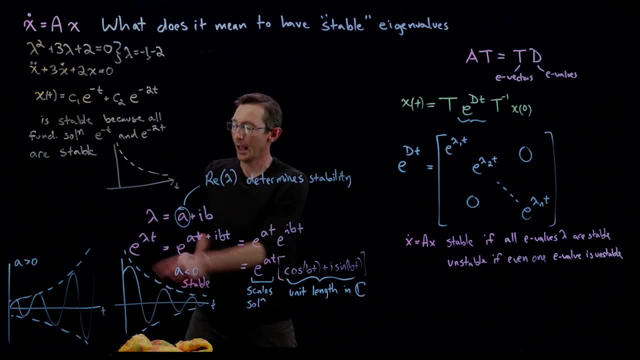 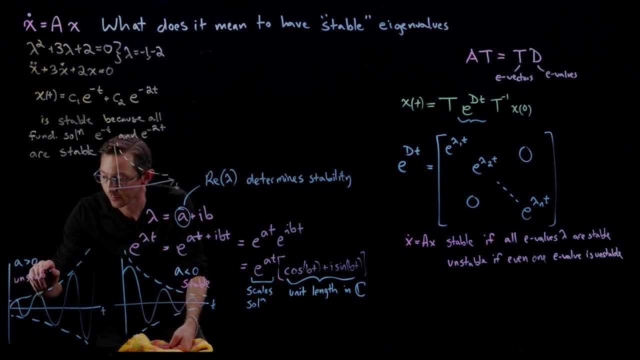 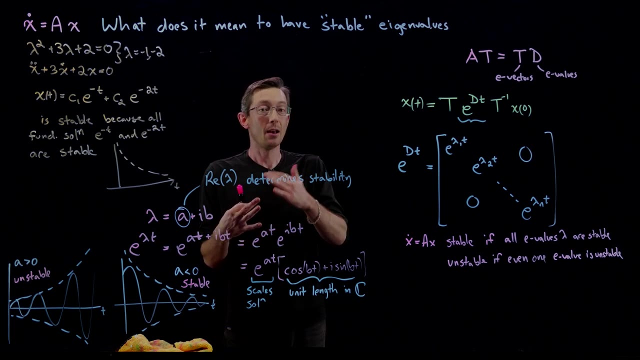 than zero is stable. a greater than zero. if my real part of my eigenvalue is greater than zero, then it's unstable, and if a equals zero. so i only have this oscillating part. we call that neutrally stable. it's. it is bounded and it's not blowing up to infinity, but it's also 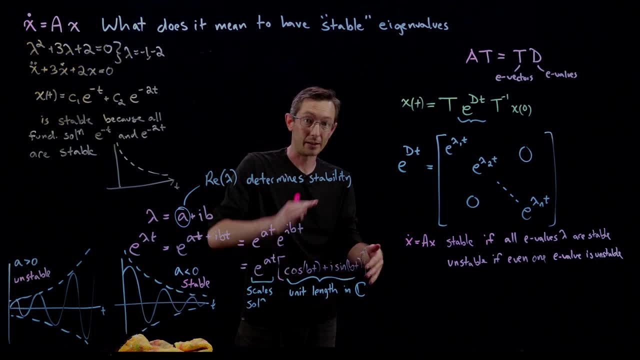 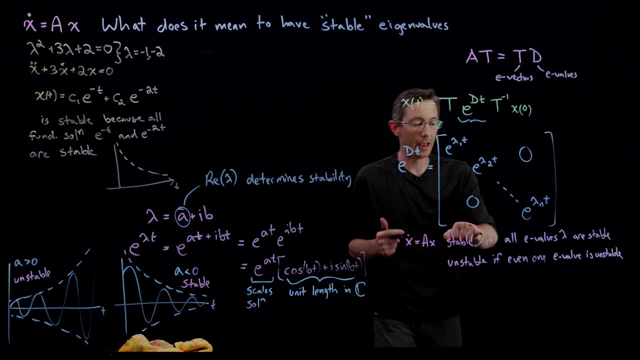 not decaying to zero, it's just kind of sines and cosines and it's going to oscillate at the same amplitude forever if a equals zero. so this is super duper important. so, and what i mean by stable here is stable, a stable lambda has negative real part. 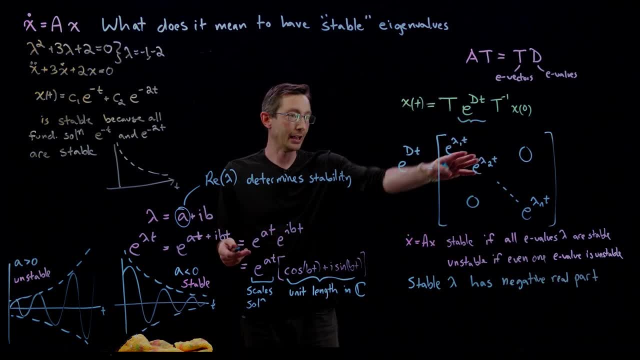 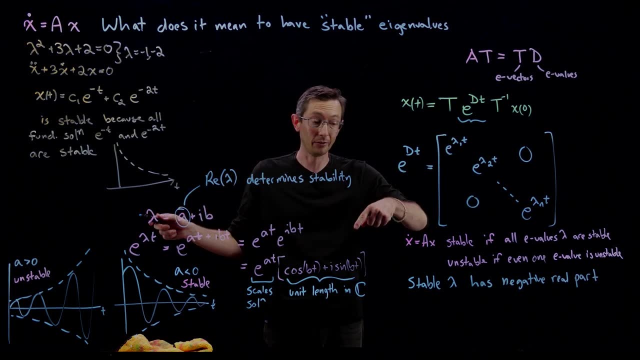 the imaginary part has nothing to do with the stability of that eigenvalue. it just causes us it to oscillate at a frequency b. but the real part of all of these lambdas have to be negative for this system to be stable. an eigenvalue lambda is stable if it has negative real part. 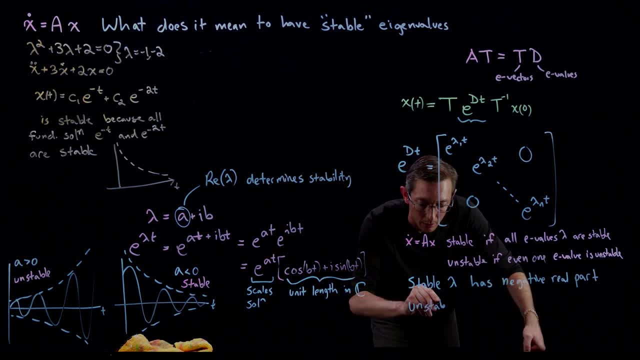 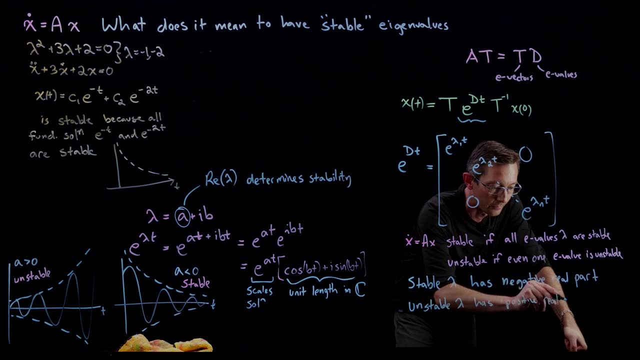 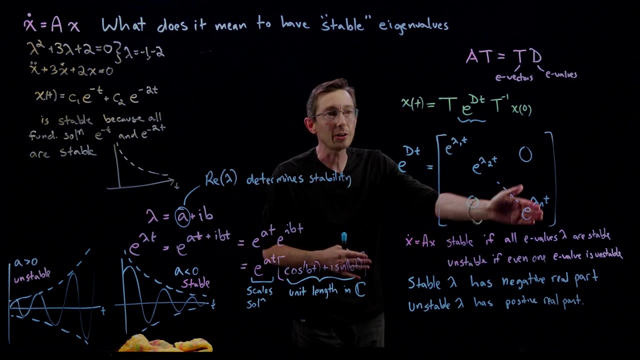 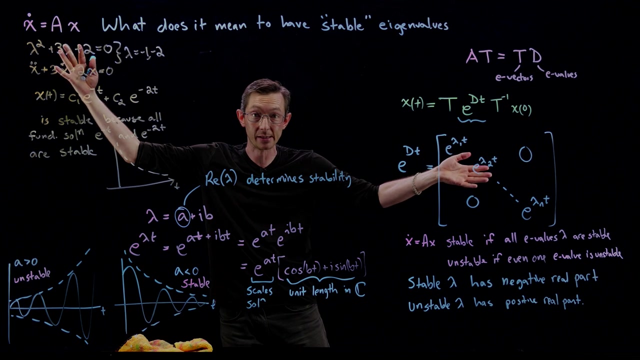 and it's unstable. an unstable lambda has positive real part in the complex plane, and so any lambda, if i have a single eigenvalue of my system, if even one of my eigenvalues of a has a positive real part, the whole system is unstable. that's how it works. 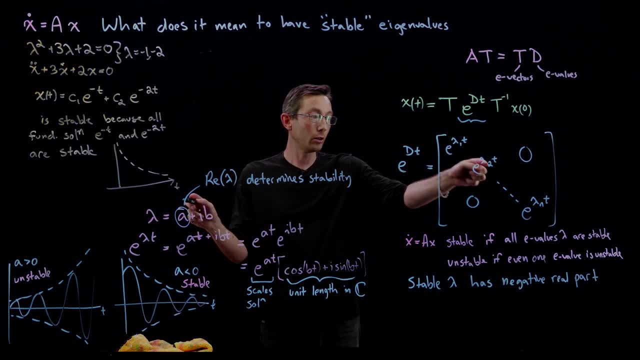 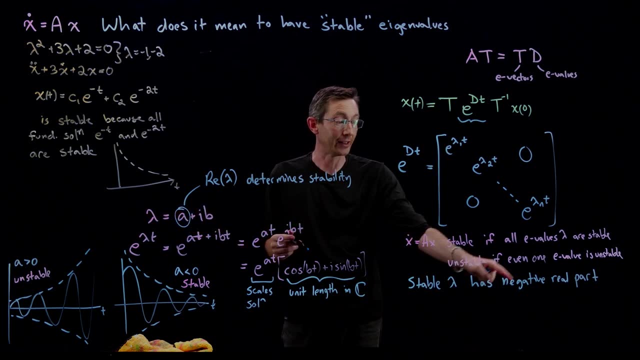 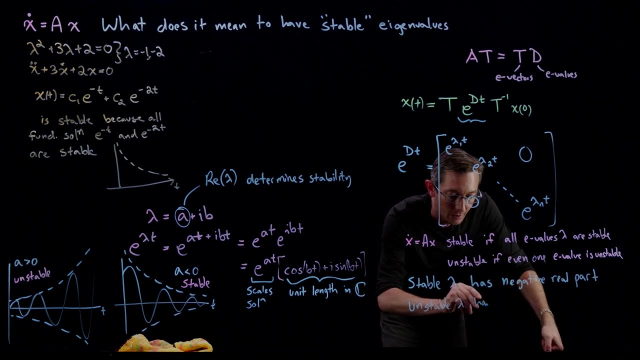 it to oscillate at a frequency B, But the real part of all of these lambdas have to be negative for this system to be stable. An eigenvalue lambda is stable if it has negative real part and it's unstable. An unstable lambda has positive real part in the complex plane, And so any lambda. 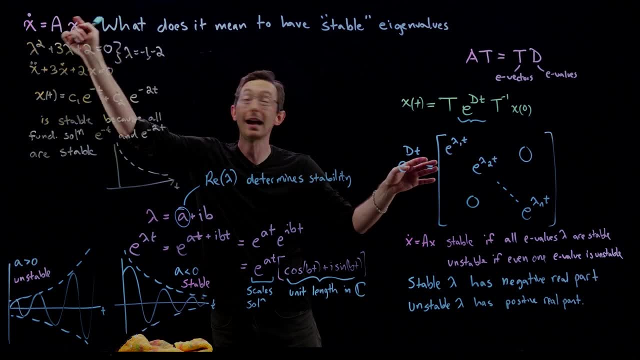 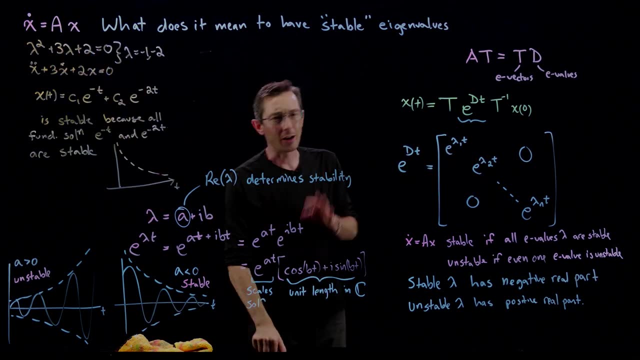 if I have a single eigenvalue, I have a positive real part, And so, any lambda, if I have a single eigenvalue of my system, if even one of my eigenvalues of A has a positive real part, the whole system is unstable. That's how it works. So I hope this kind of clears it up for you. I'm going to use this. 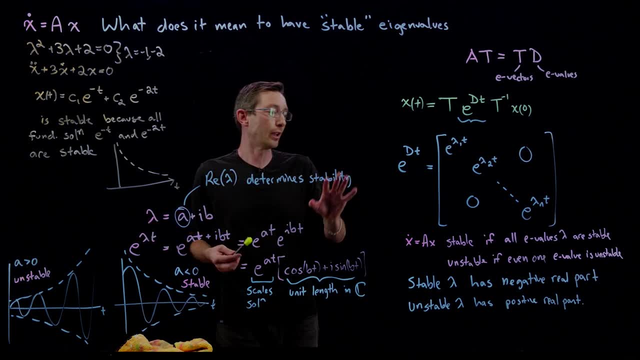 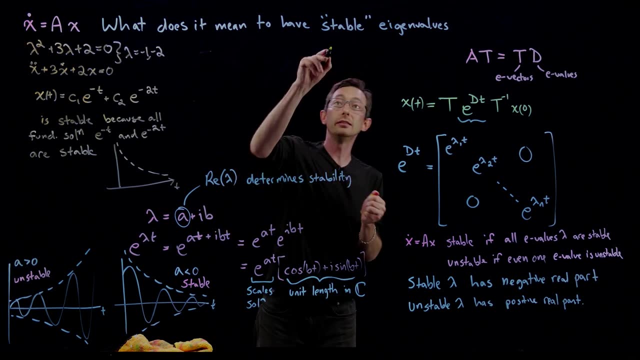 terminology like you're going to hear it so many times. Don't make a drinking game out of me talking about stable eigenvalues, And I wanted you to know what I meant by that. And so, literally, if I plot my eigenvalues in the complex plane, so here's the complex plane And let's say I've got a bunch of 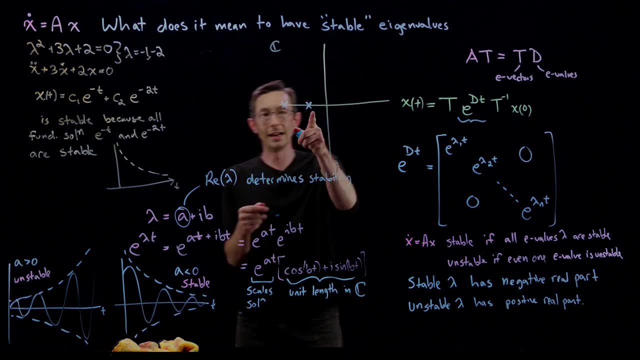 eigenvalues and I've got negative real part And I've got negative real part And I've got negative one, negative two, nice and stable. nice and stable. I've got negative 1.7 plus I negative 1.7. 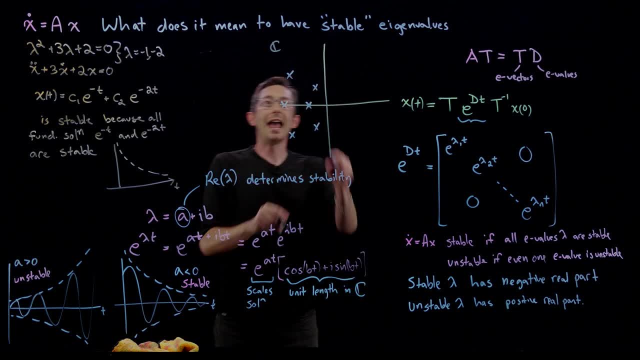 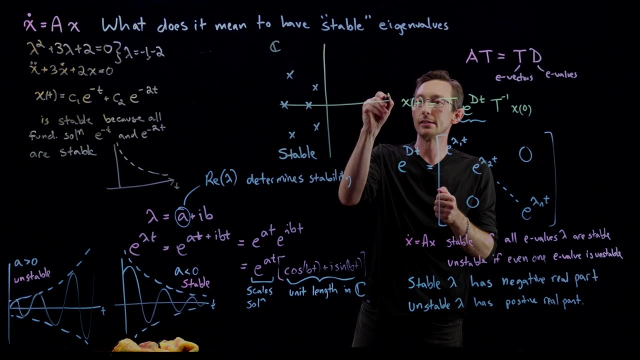 minus I. I've got a bunch of stable eigenvalues. Any eigenvalue in this left half plane is stable. This is called the stable left half plane because if eigenvalues live in this plane where the real part, these axes- sorry, I should draw the axes. This is the real part of lambda and this is the. 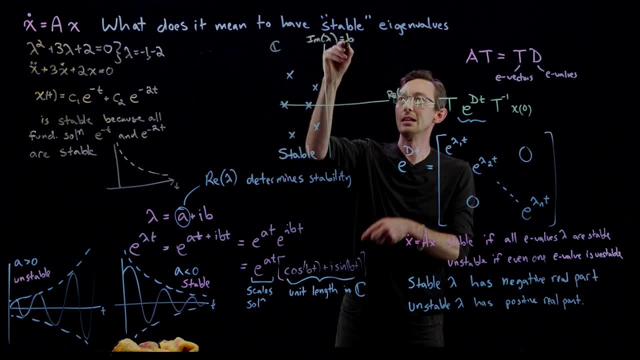 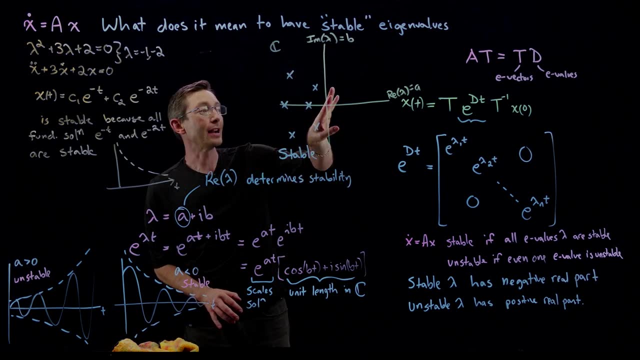 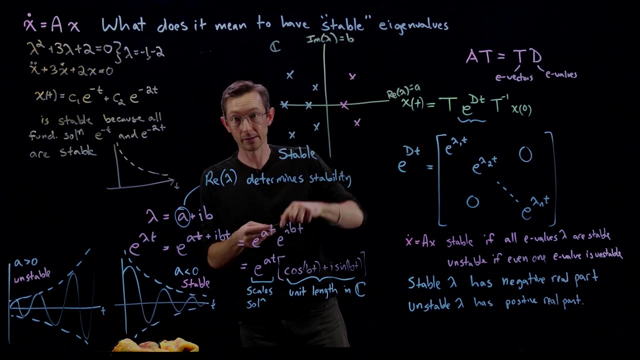 primary part of lambda, which I've called- you know B here and I've called A here. If my real part is negative, all of these eigenvalues are stable. And if my real part is positive, if I have an eigenvalue out here or here, these are unstable eigenvalues. okay, So I have the stable left half. 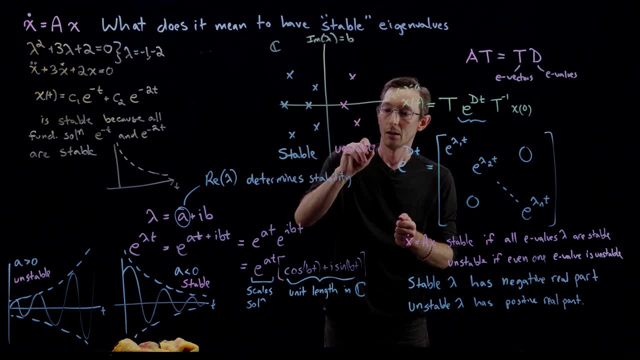 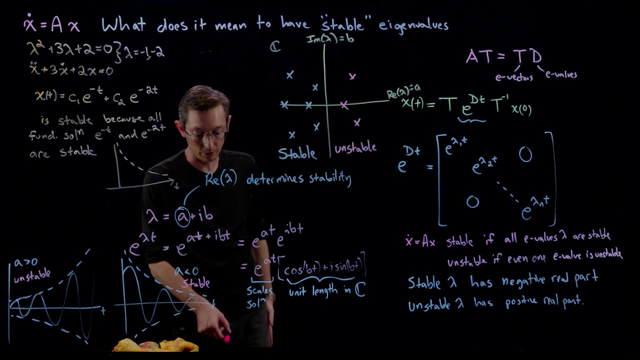 plane and the unstable right half plane And this is going to come up a bunch in control theory. We call these poles of a system Control theory, you know, but they're really just the lambdas, the roots of my sorry, the. 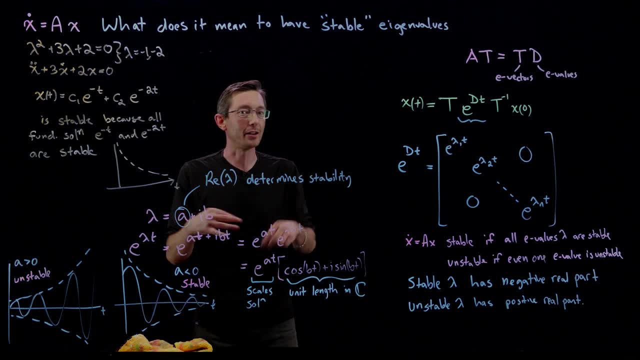 okay, so i hope this kind of clears it up for you. i'm going to use this terminology like you're going to hear it so many times. don't make a drinking game out of me talking about stable eigenvalues. and i wanted you to know what i meant by that. and so, literally, if i, if i plot my eigenvalues in the complex plane. 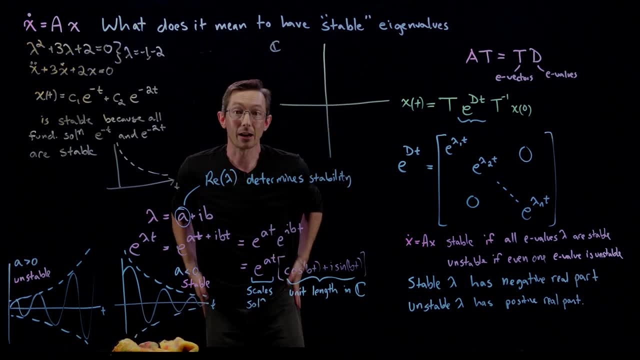 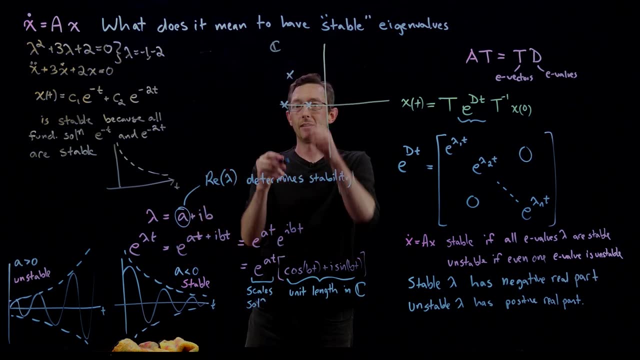 so here's the complex plane and let's say i've got a bunch of eigenvalues and i've got, you know, negative one, negative, two, nice and stable, nice and stable. i've got, you know, negative 1.7 plus, i negative, 1.7 minus. i've got a bunch of stable eigenvalues, any eigenvalue in this left half plane. 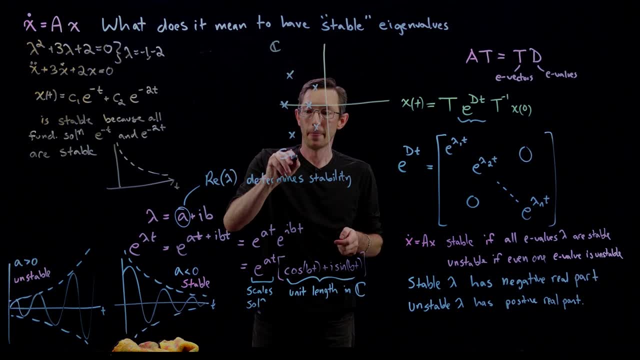 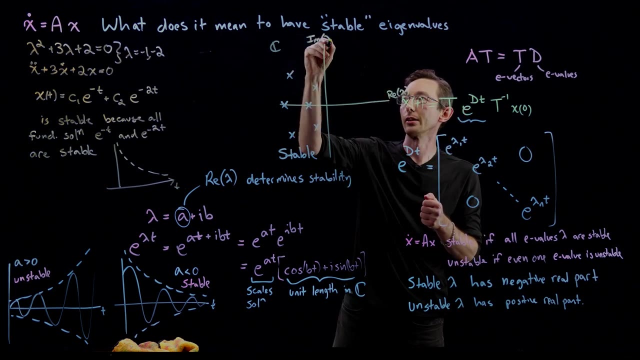 is stable. this is called the stable left half plane because if eigenvalues live in this plane, where the real part, these actual eigenvalues are the real value for us- Sorry, I should draw the axes. This is the real part of lambda And this is the imaginary part of lambda which I've called, you know, B here. 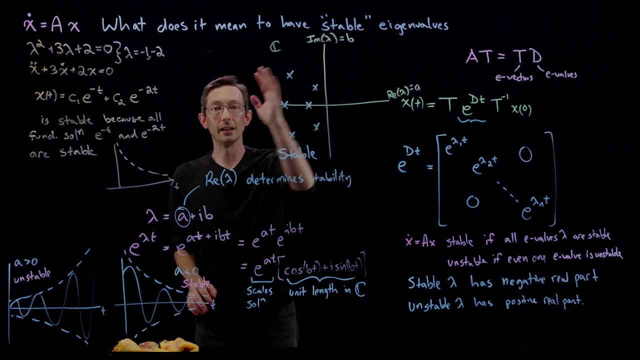 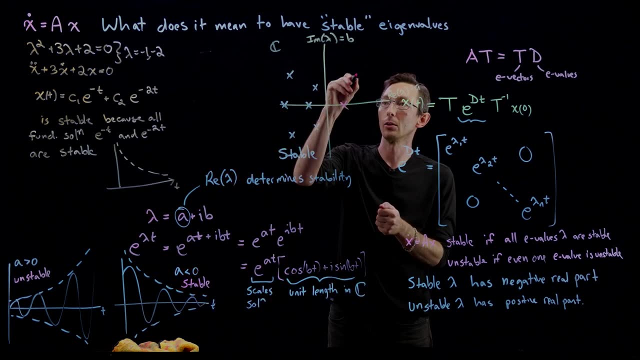 And I've called a here- if my real part is negative, All of these eigenvalues are stable. and if my real part is positive, if I have an eigenvalue out here or here, These are unstable eigenvalues. Okay, so I have the stable left half plane and the unstable. 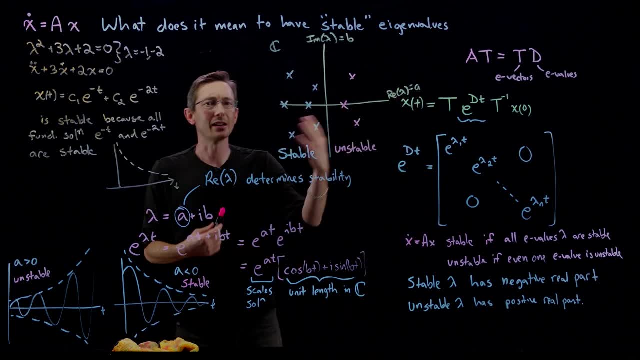 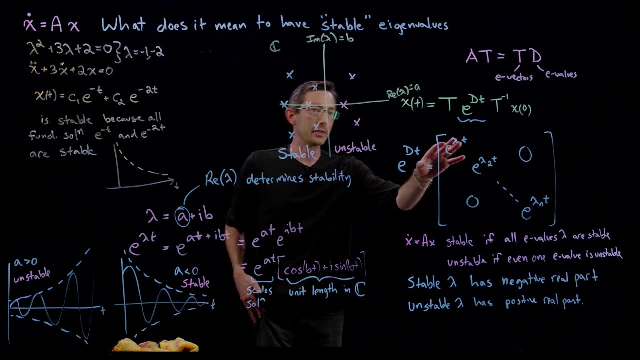 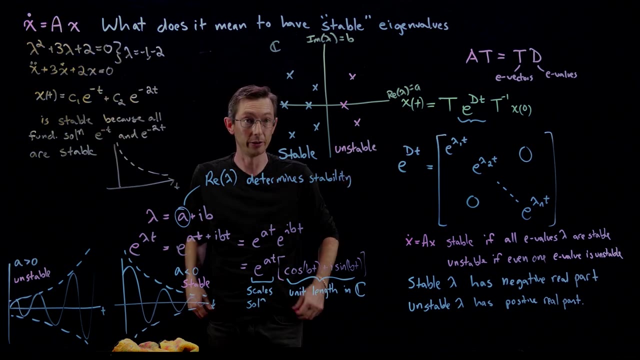 Right half plane and this is going to come up a bunch. in control theory We call these poles of a system in control theory, you know, but they're really just the lambdas: the roots of my- Sorry, the eigenvalues of my- a matrix, or the roots of my characteristic polynomial. 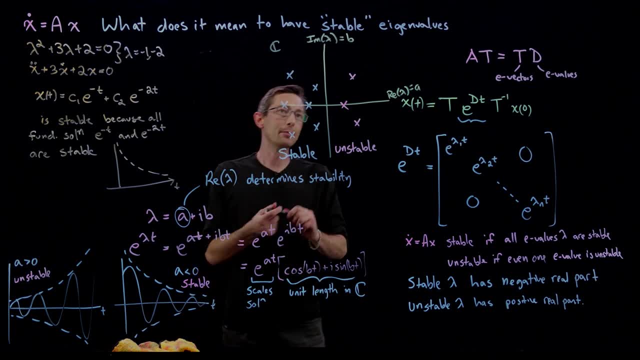 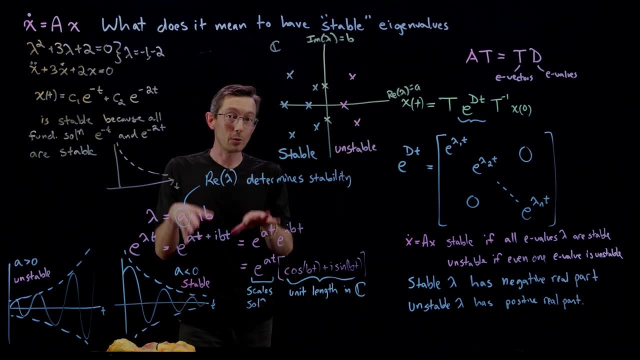 And this is how we define stability. and, similarly, any points here are neutrally stable. If they're perfectly on the imaginary axis, they're neutrally stable. Okay, I really wanted you to see that, because I, I, I, I need you to have this kind of deep intuition and gut feeling of what it means for an eigenvalue to be stable, and 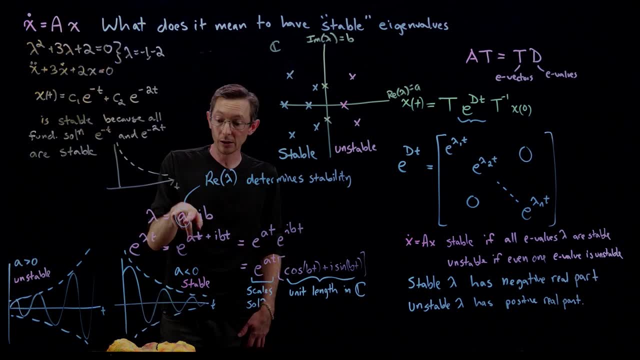 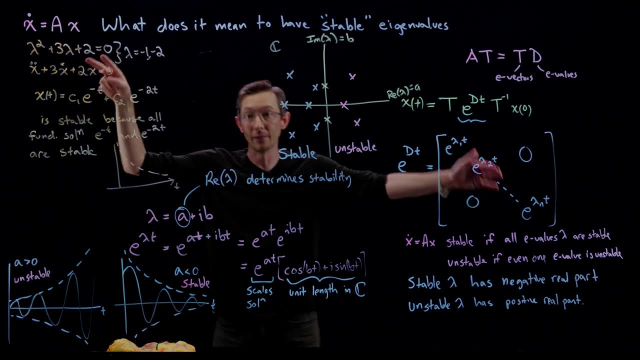 Eigenvalue of this, a matrix, is stable if it's real part is negative and it's unstable If it's real part is positive. and for a system, I need all of the eigenvalues to be stable for this system to be stable. All right, Thank you. 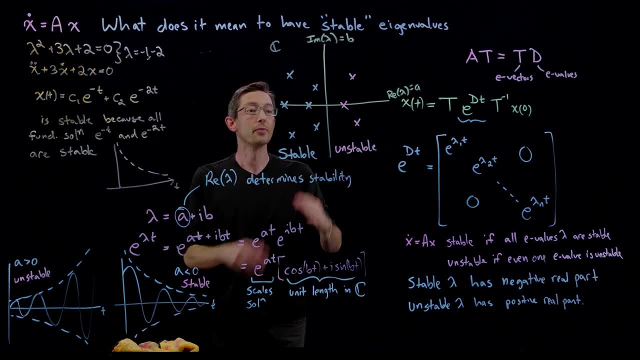 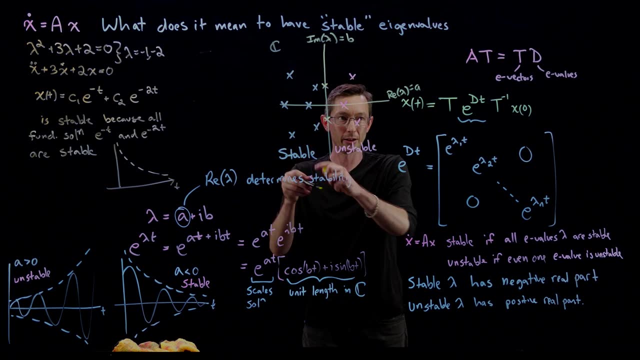 eigenvalues of my A matrix or the roots of my characteristic polynomial, And this is how we define stability. And, similarly, any points here are neutrally stable. If they're perfectly on the imaginary axis, they're neutrally stable. Okay, I really wanted you to see that, because I need you. 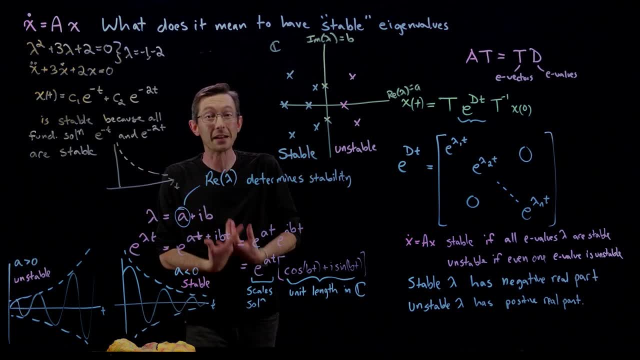 to have this kind of deep intuition and gut feeling of what it means for an eigenvalue to be stable, An eigenvalue of this. A matrix is stable If its real part is negative and it's unstable if its real part is positive. And for a system I need all of the 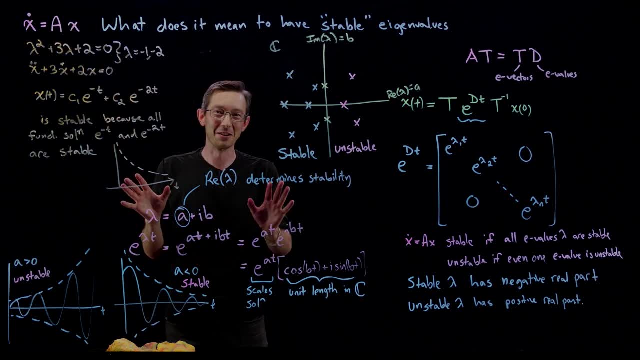 eigenvalues to be stable. for this system to be stable, All right, thank you. 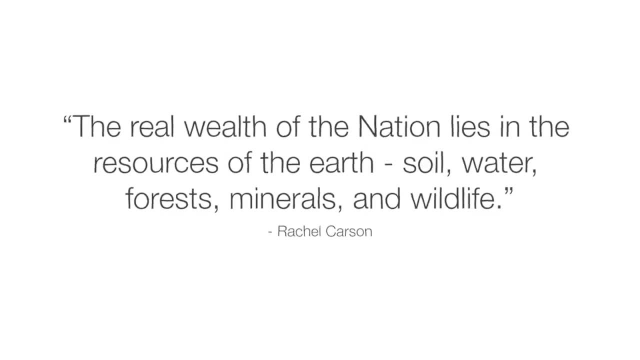 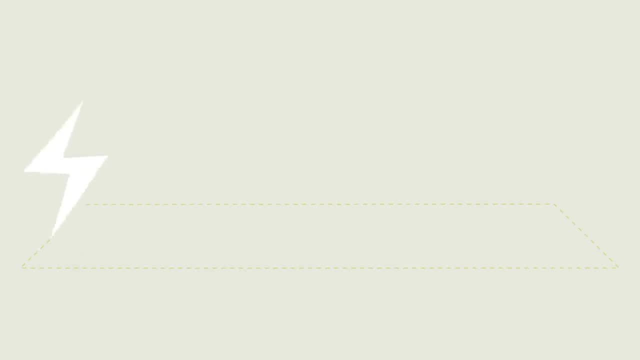 No matter how we make electricity, it takes up space. Electricity from coal requires mines and plants to burn it and convert the heat into electricity. Nuclear power takes uranium mines, facilities to refine the uranium, a reactor and a place to store the spent fuel safely. 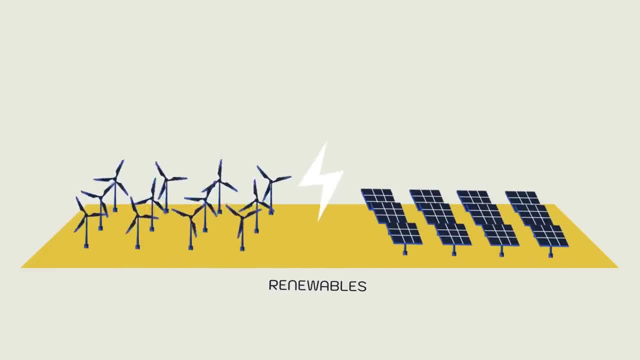 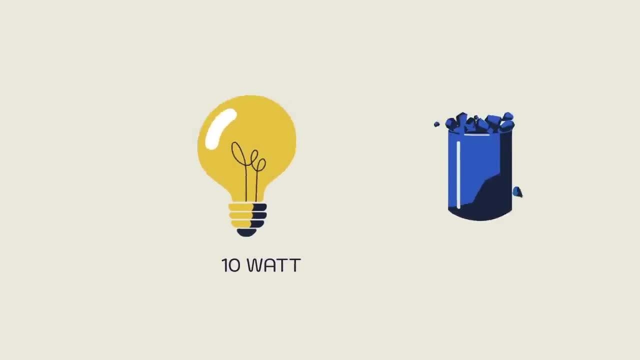 Renewable energy needs wind turbines or solar panels. How much space depends on the power source. Say you wanted to power a 10-watt light bulb with fossil fuels like coal. Fossil fuels can produce up to 2,000 watts per square meter. 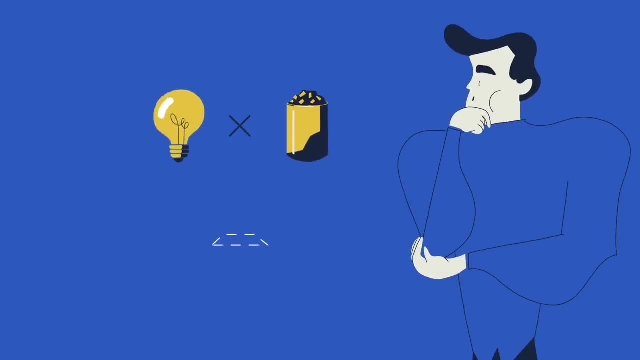 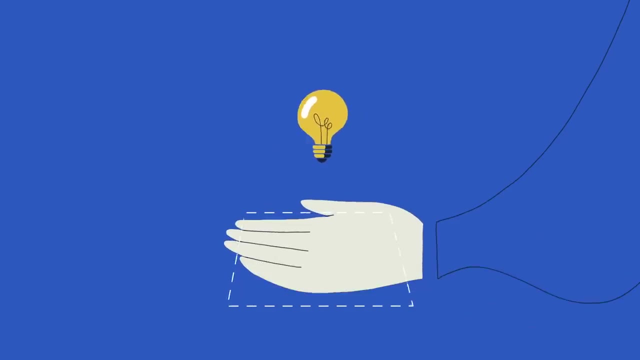 so it would only take a credit card-sized chunk of land to power the light bulb. With nuclear power, you might only need an area about the size of the palms of your hands. With solar power you need at least 0.2.. 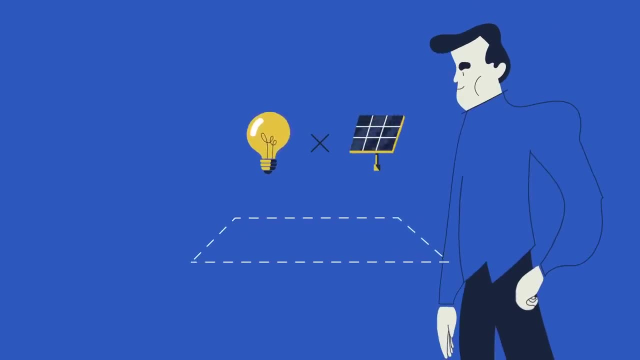 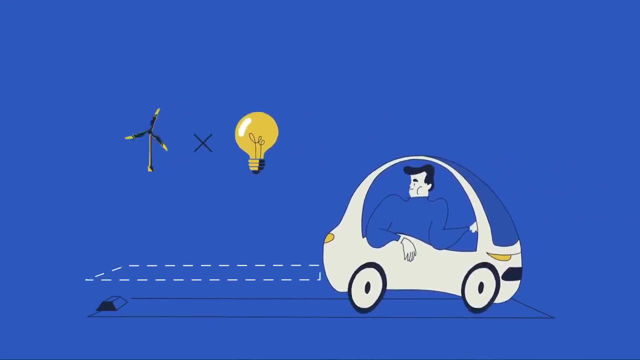 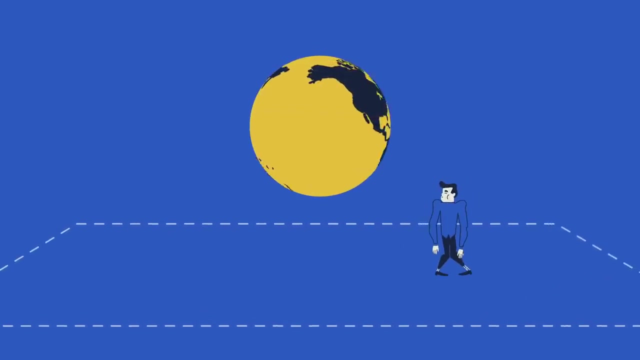 That's 1.3 square meters of land, twice the size of a cafeteria tray. Wind power would take roughly 7 square meters, about half the size of a parking space, to power the bulb, When you consider the space needed to power cities, countries and the whole world. 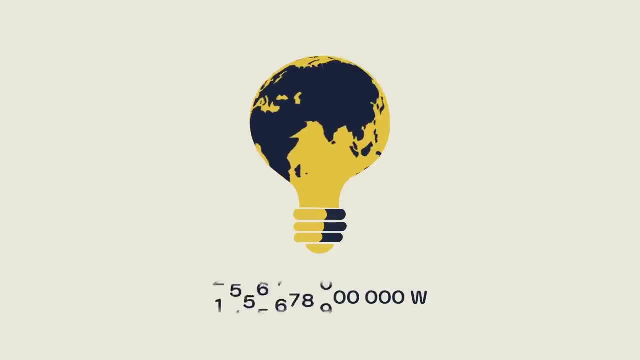 it adds up fast. Today the world uses 3 trillion watts of electricity. To power the entire world with only fossil fuels, you'd need at least about 400 square kilometers of space, roughly the area of Grand Bahama Island. With nuclear energy, you'd need almost four times as much space. at a minimum.